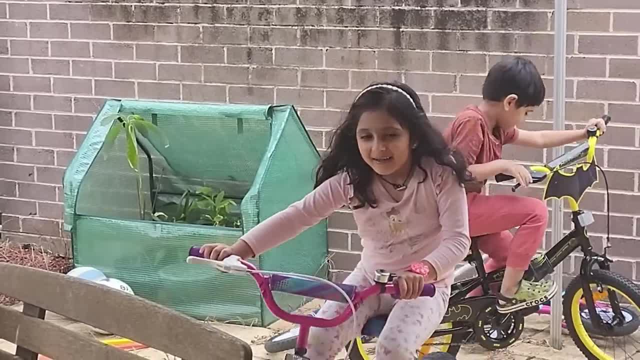 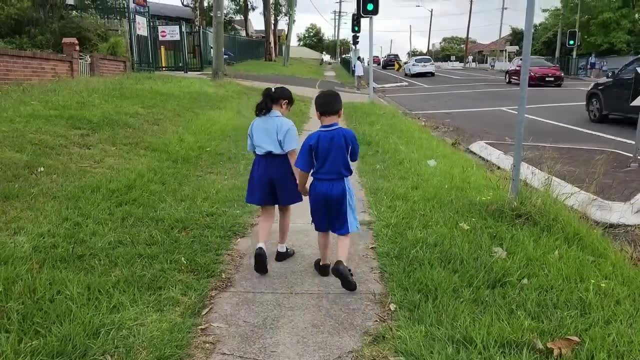 The video we are going to watch today is from the video that we saw in the previous video. This is a video that we saw in the previous video. It's a video that we saw in the previous video. I'm looking forward to seeing what it's like to be a teacher. 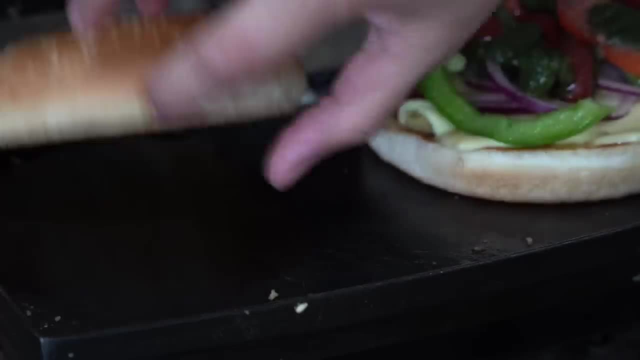 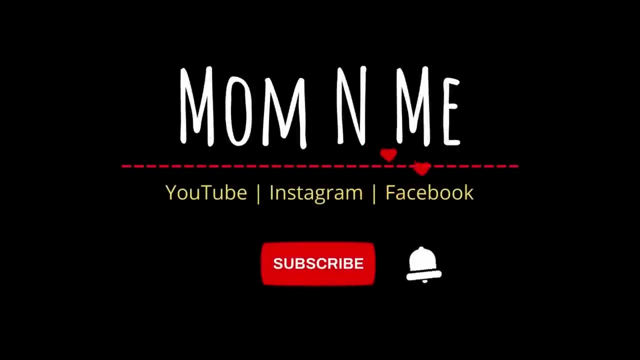 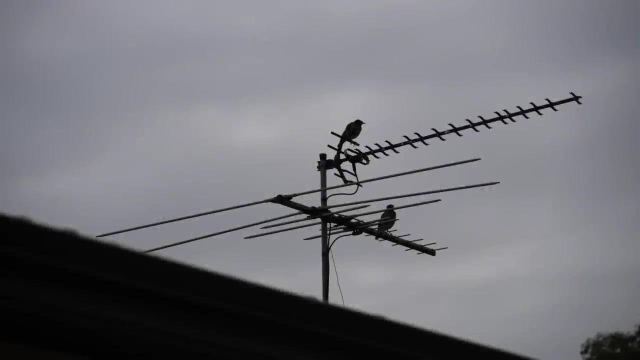 I'm going to teach you how to make a simple and easy video If you have a lot of time and energy. I hope you enjoy it. hi guys, i hope you all are doing great. with the start of the new year, i have started a new routine. 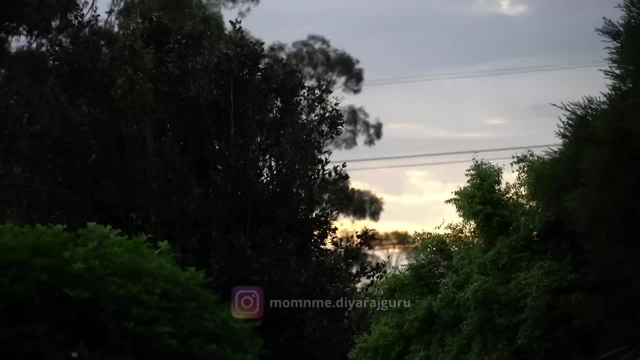 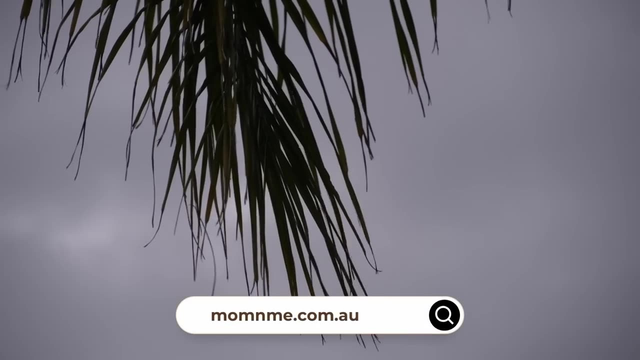 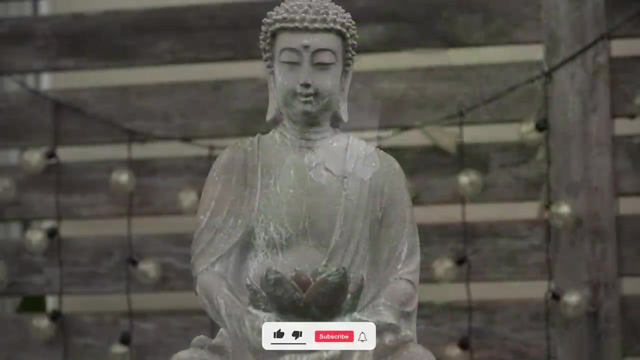 for myself. i had made few new year's resolutions for myself at the beginning of year 2023 and my new routine is based on to achieve these new year's resolutions. so, firstly, what i did was to write down all the things that i wanted to achieve in 2023 or years coming ahead, having a 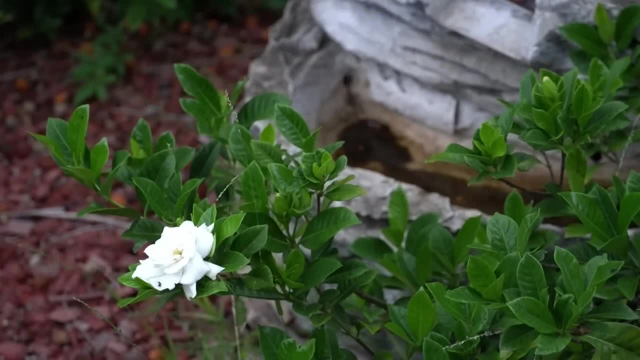 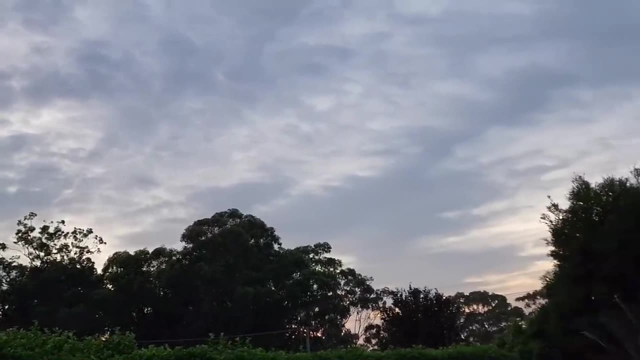 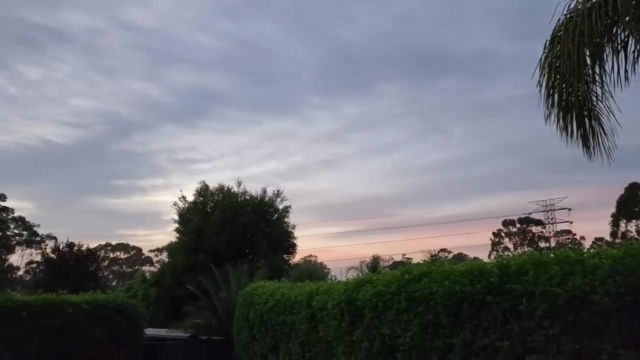 list makes it more concrete. next, i converted my targets into doable or actionable items and made a daily to-do list, and from there on, i take some action each day to achieve my long-term goals. simple, isn't it? well, it sounds very cliche, but let's put it into perspective. so one of my goals: for year 2023 is to focus on my physical and inner development and well-being, and i concluded that these four things i need to do to achieve my new year's resolutions for myself at the beginning of year 2023 are the things that i need to take care of, and it's in order of their importance. the first 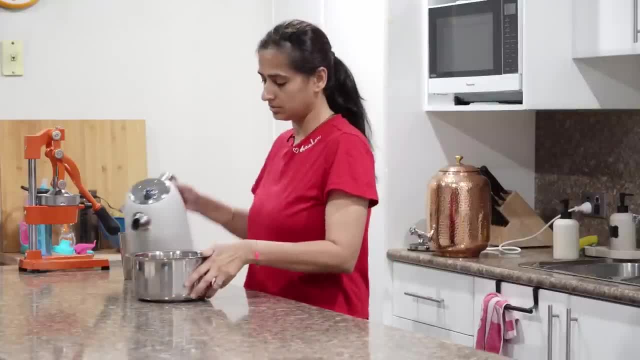 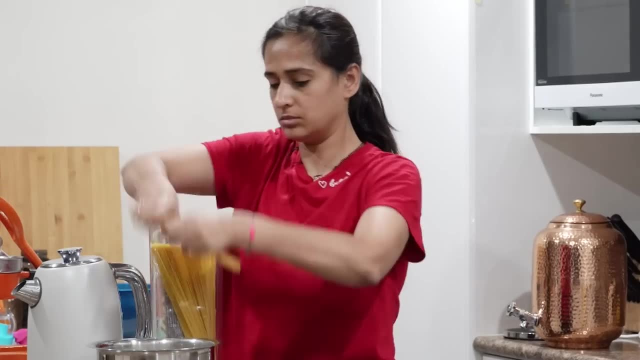 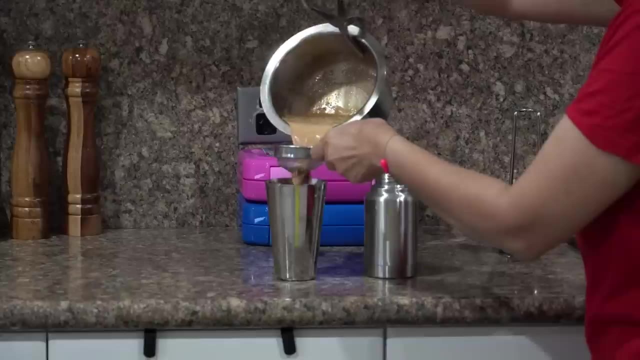 one is physical health, second is mental health, third is spiritual health and lastly, financial health. so, first and foremost, the most important thing for me is my physical well-being being fit and healthy, and nothing to do with my weight or shape, purely being able to function better. 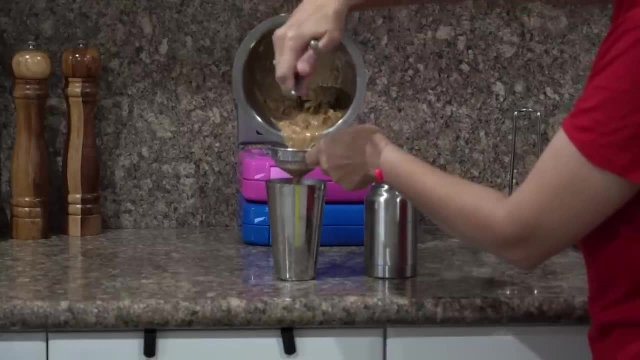 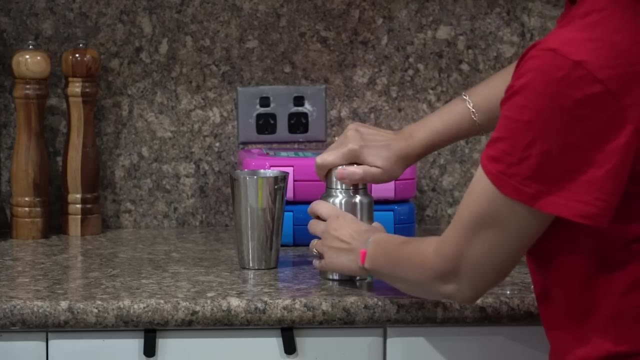 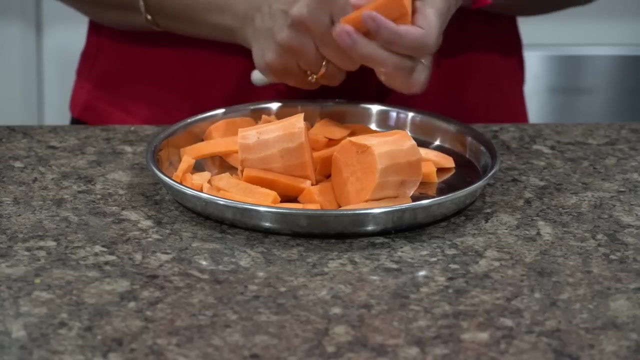 and for that i know i just need to prioritize myself and also be consistent with what i'm doing, that is, going to the gym. i have been going to the gym since a year now but honestly i have never been consistent because i've always given more importance to either buying weekly grocery 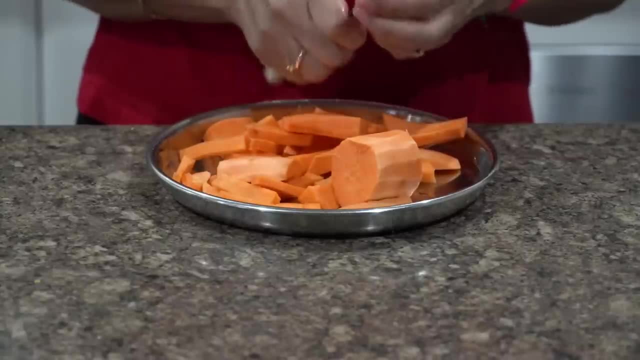 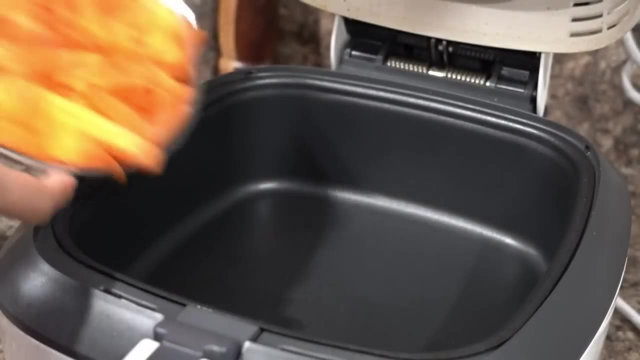 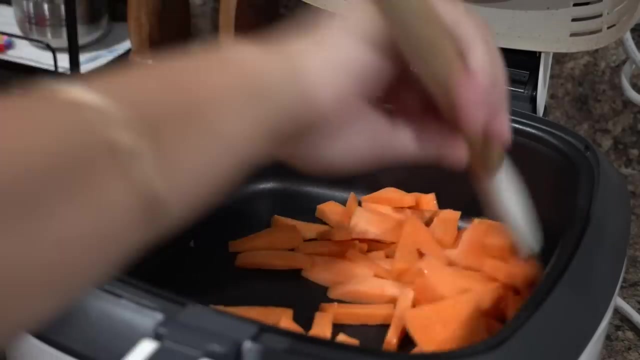 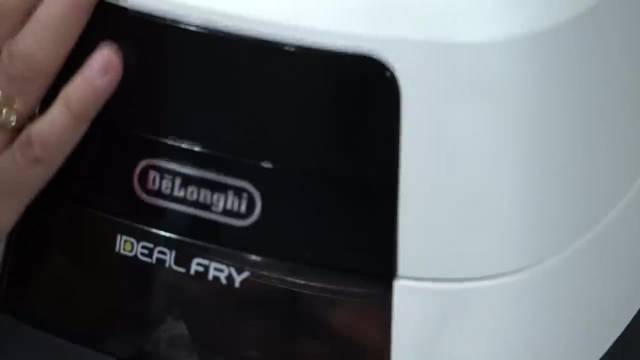 or shooting or editing a video or cooking food time, consuming food for my kids and my family and not prioritizing myself, my health, and i bet most of you guys are doing the same. we, as mothers, want to keep everyone around us happy, even if it means sacrificing our own needs, but we need to understand that self-care is not self-indulgence. self-care is an act of survival, god forbid. but what if you are chronically sick tomorrow or something else happens to you? the world will not stop, it will go on even if you are sick. so taking care of yourself first is unquestionably a priority which i have understood now so being 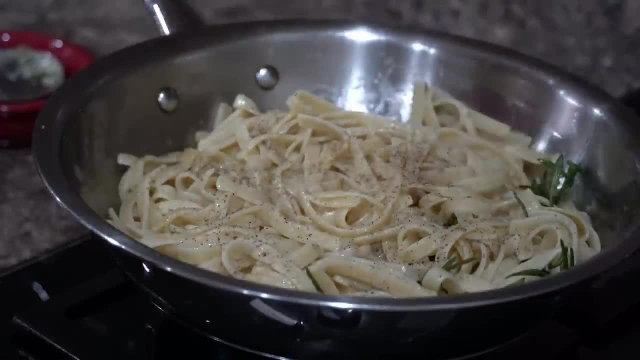 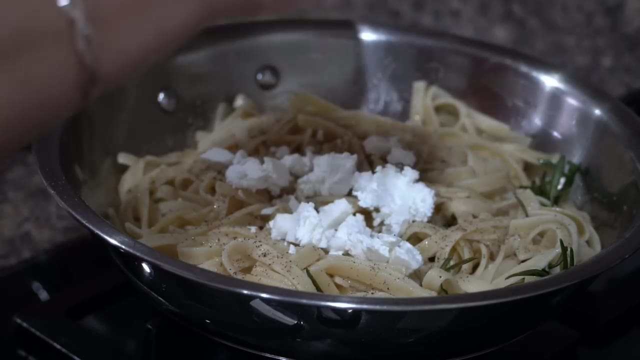 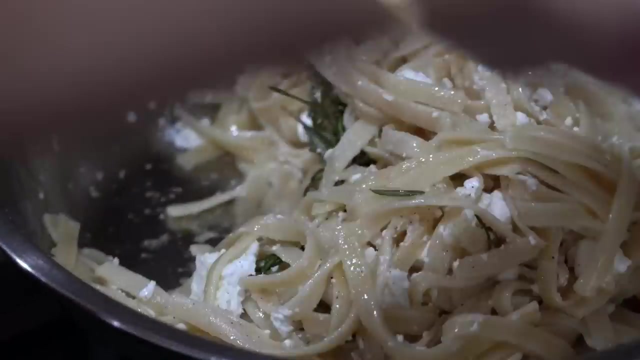 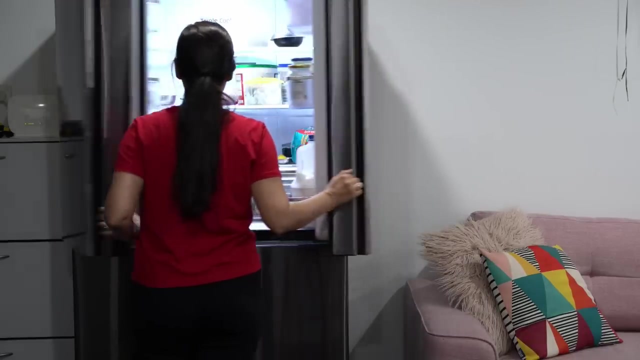 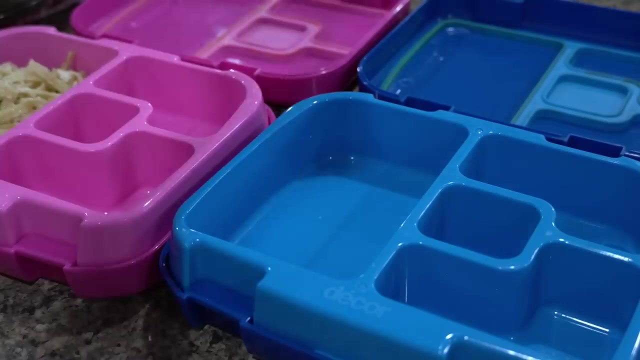 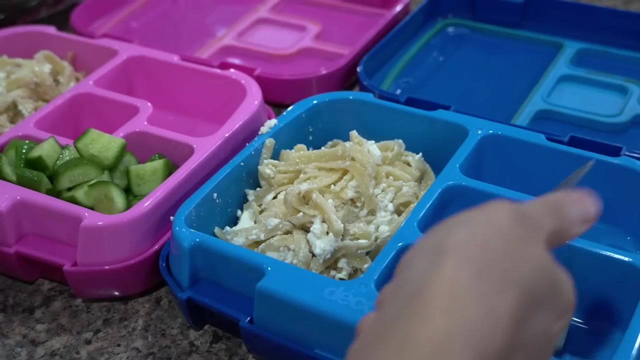 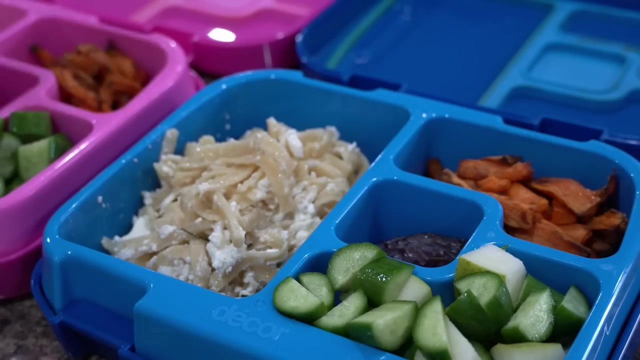 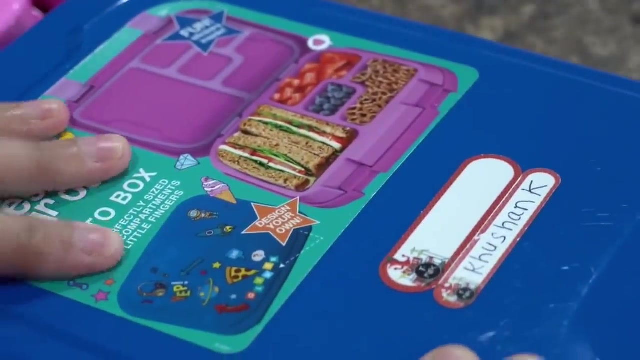 fit is my resolution, and going to the gym on daily basis is my action to achieve my long-term goal. by the way, i take a break on wednesdays. i try to go four times a week, unless something urgent comes up while you can, let me know at all. 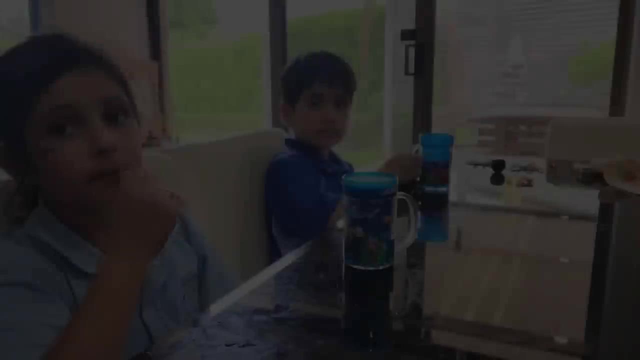 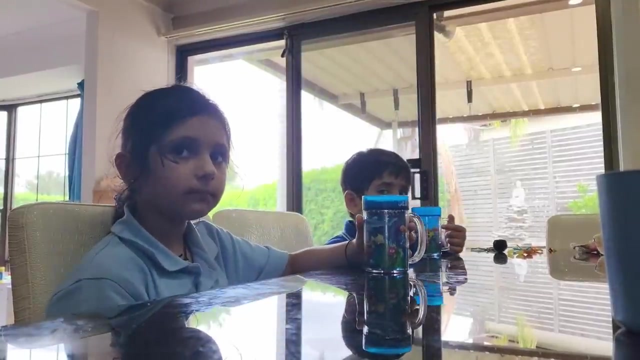 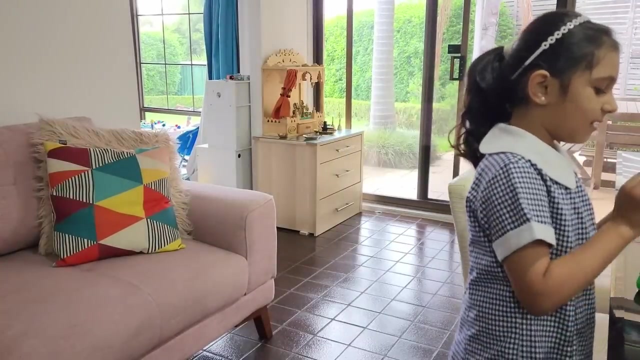 false bond. i'm worth something more, for sure. H könig, a mom girl, a mom, you experience immense stress taking care of kids. i am sure most of you would relate. being a mom is challenging, as you're constantly being interrupted. sometimes we lack control of the situation. 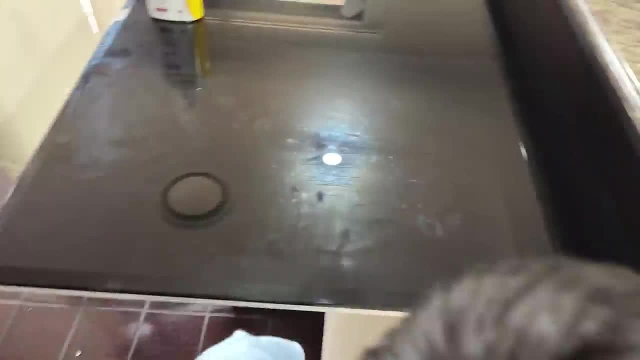 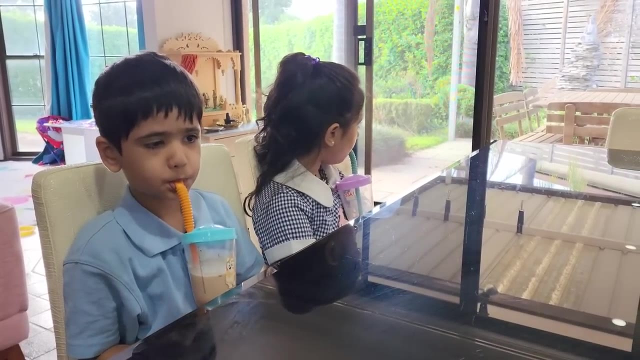 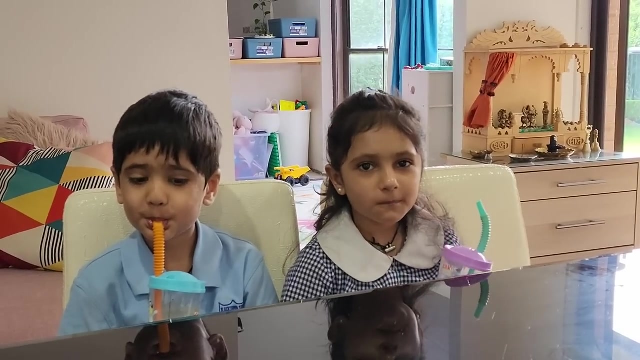 having tantrum cries from our kids in middle of something important pretty much. we have a lot of emotions involved and cortisol spikes leading to stress. also as a mother, sometimes we tend to help our kids more than they need and thus they become dependent on us. i'm a culprit to that as well. 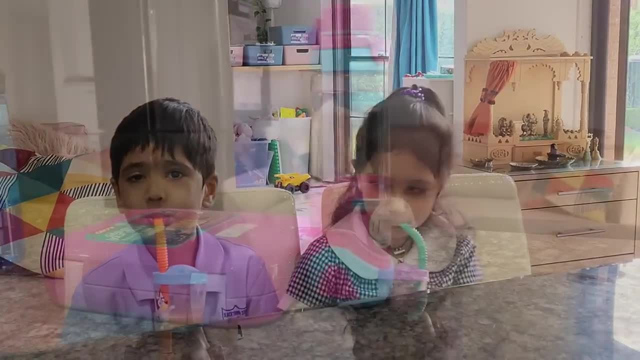 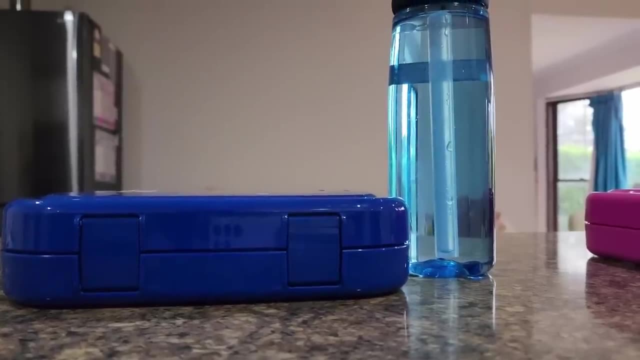 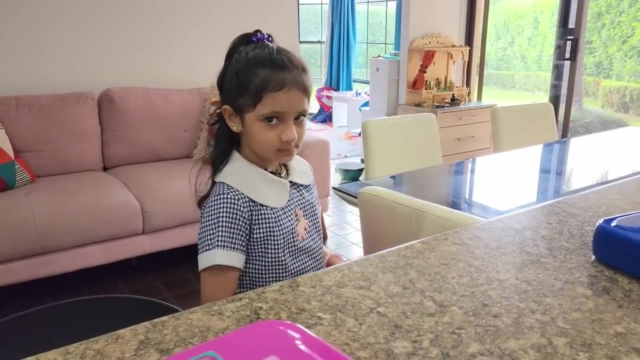 sometimes, when we are rushing to get them out of the door, we quickly make them wear clothes, jackets, shoes, etc. etc. i used to do the same and realized that they didn't want to do things on their own, even on a holiday. they wanted my assistance in everything, which was very draining. 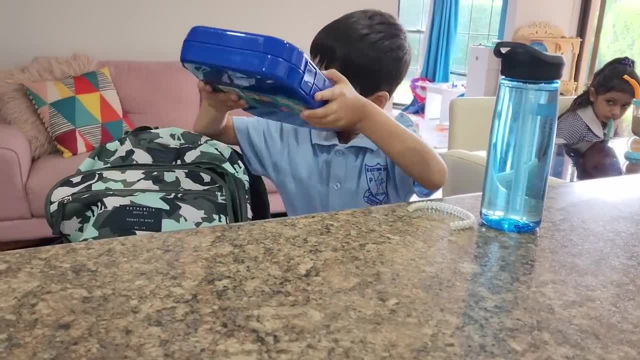 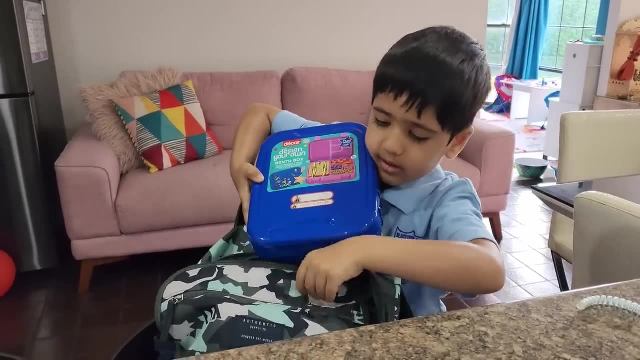 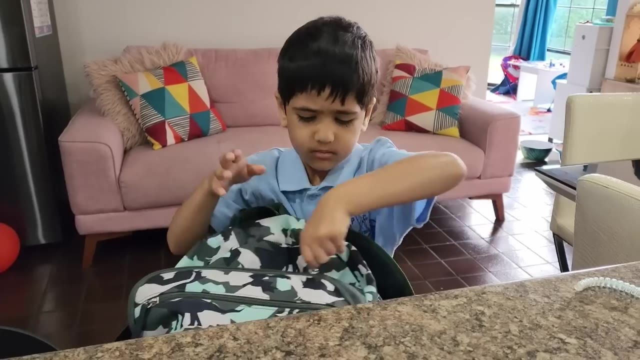 for me, especially mentally. so i decided that once we are back into the school routine, i will wake them up 15 to 20 minutes early and let them do their things. previously, every morning was a rush or a juggle to get them to school on time because i was in charge of getting kids ready. 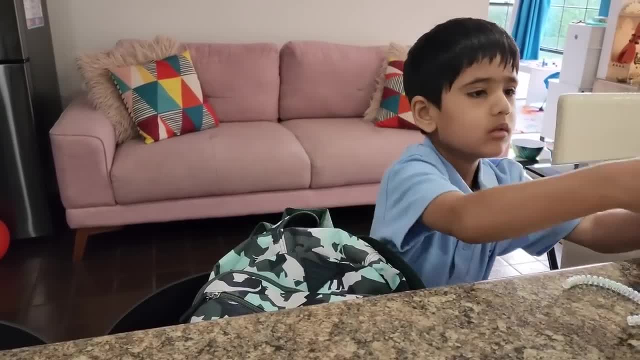 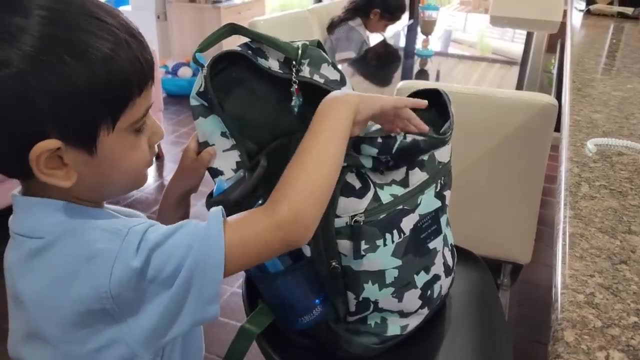 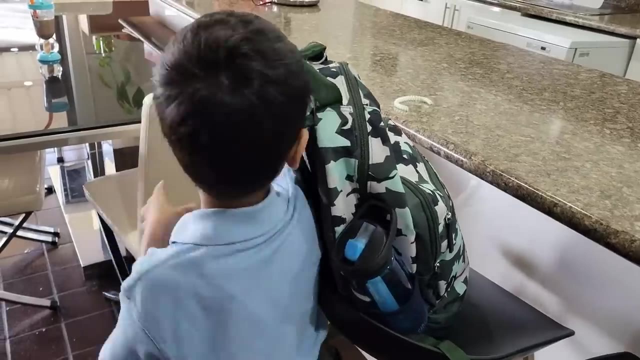 but now i have made them in charge of getting themselves ready. they brush their teeth themselves, dress themselves from clothes to socks, to hair, to wearing shoes, pack their bags and check if they have raincoat, their folder and other necessary things in their school bags. they come back home. 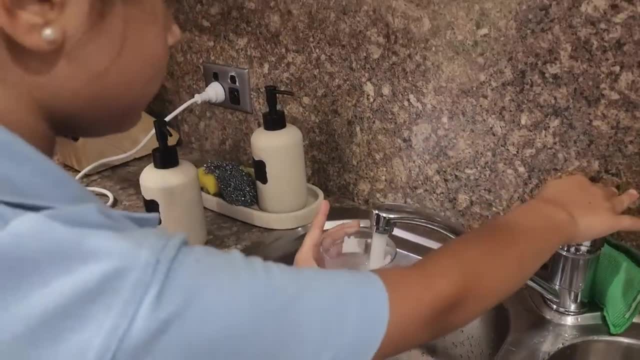 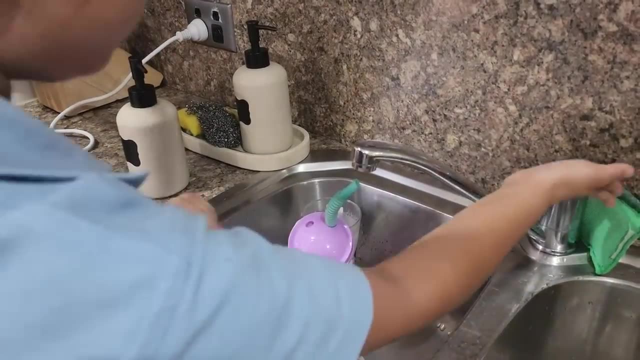 and unpack their bags, put the tiffin box in the sink for me to clean up and if there is a note from the teacher they would hand it over to me. they take shower themselves with my minimal need. but yes, they do need a little assistance with that. but i'm sure they will get independent. 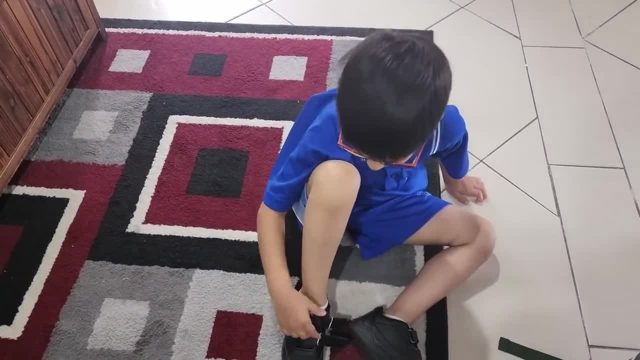 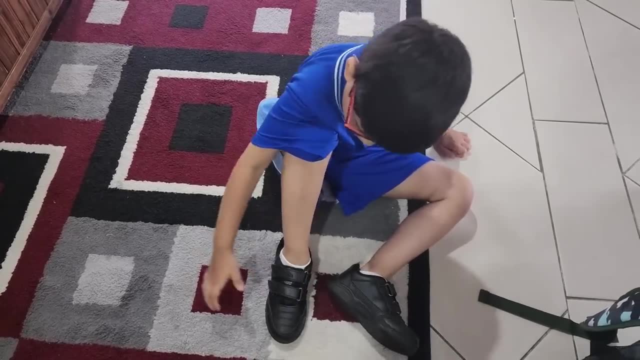 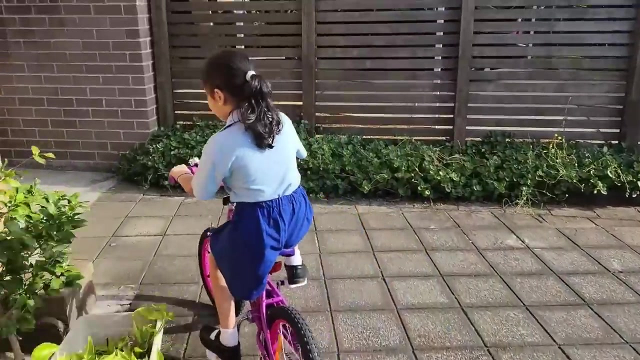 just bringing these few changes has relaxed my mind, as previously i used to be after them- you to get ready, as in their head, it was my job. now kids think it's their job and they have to do it. in fact, dhyani once mentioned, while packing her bag in the morning, that mama once i get my task. 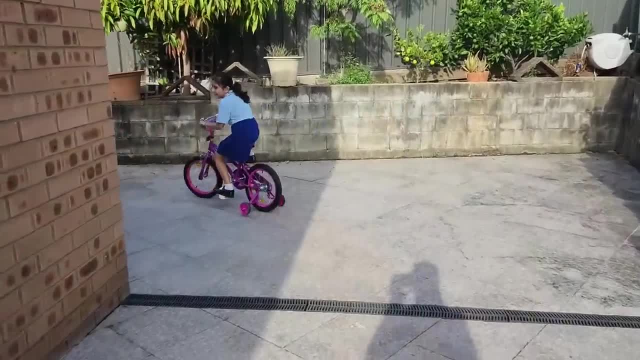 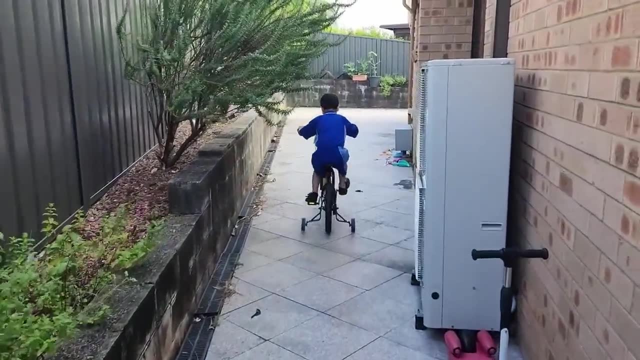 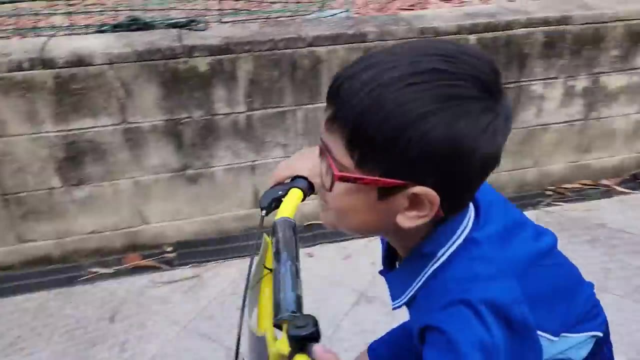 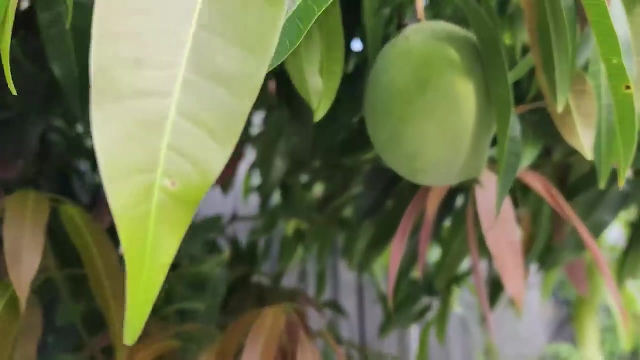 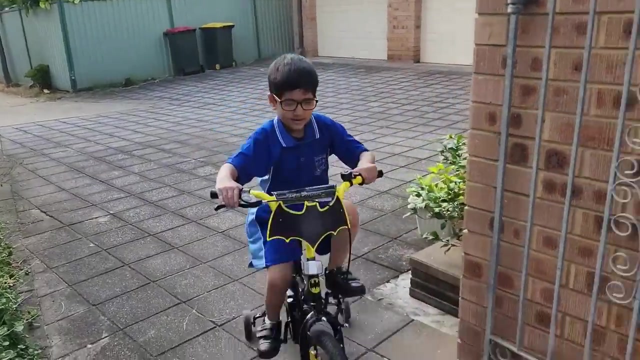 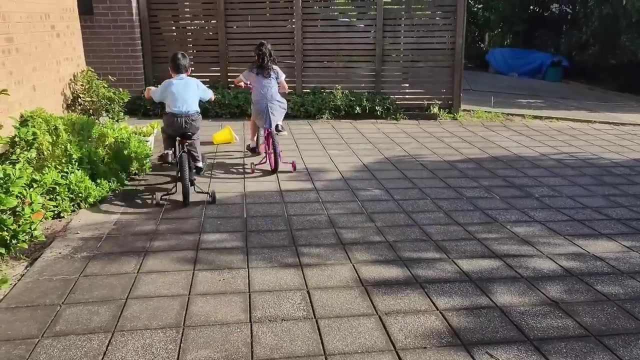 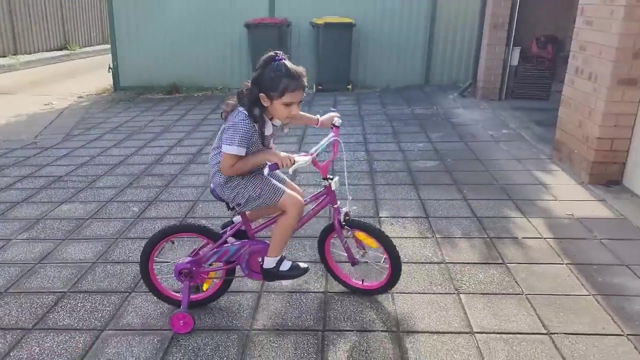 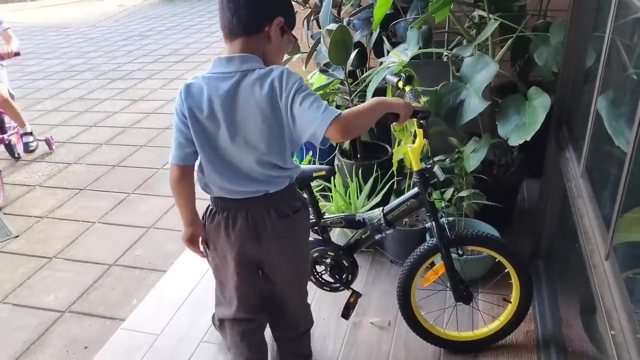 out of the way. i feel much relaxed and i can play freely, otherwise that one outstanding job keeps creeping in my head. i was like: welcome to mama's world, child. so i'll let mama back u right now, hi. so what, oh dude, Oh Hoo Ha, If you hide your fluttering heart? 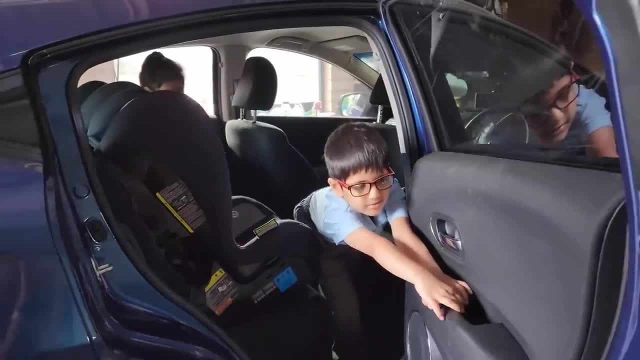 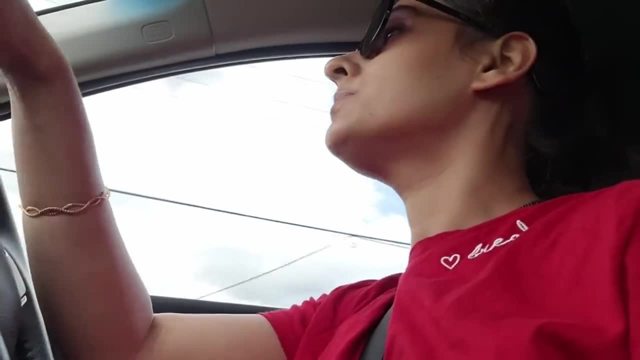 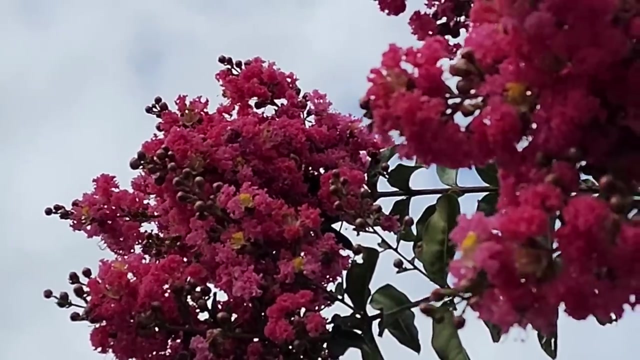 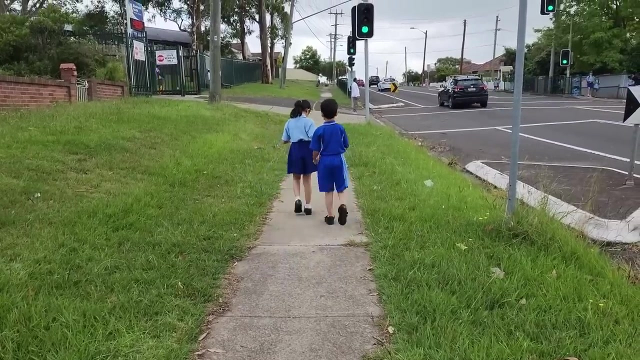 It becomes a double-edged sword. The burning heart: It's burning more. The longing for you: It's piling up. and I'm about to. What do I do? I don't know how to do it. I feel like I'm going to be different. I feel like I'm going to be different. 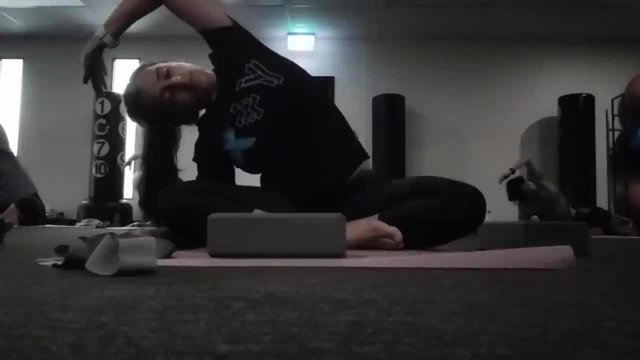 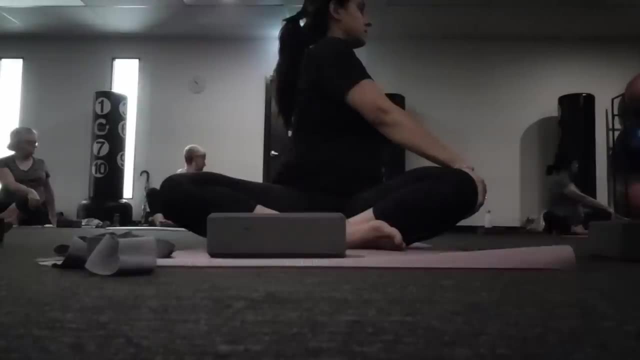 I feel like I'm going to be different. Another thing I do is that I have started taking relaxing yoga classes, which is part of my gym membership. Previously, I used to not attend this class as I only wanted to be slim and would rather prefer to run on the 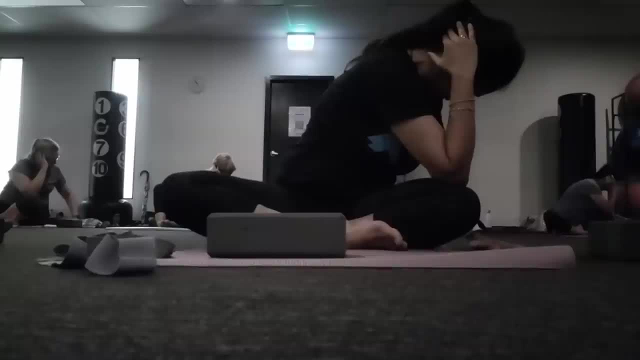 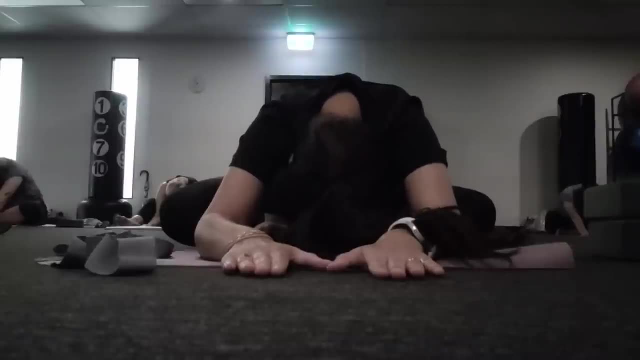 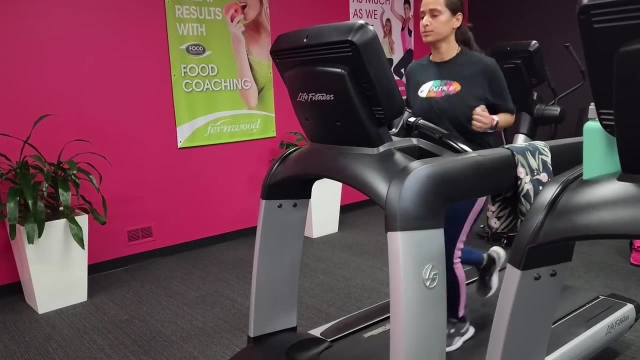 treadmill than do yoga, but now I do take this class to relax my mind. This is a full house class and each and every person is so rejuvenated and relaxed after taking self-care Thursday yoga session, so even I have made it a priority now. Another change I made was doing online groceries. 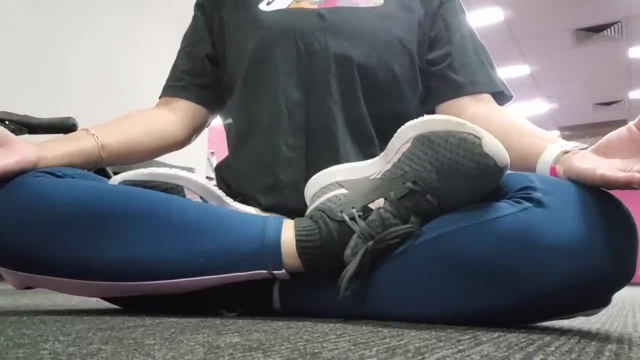 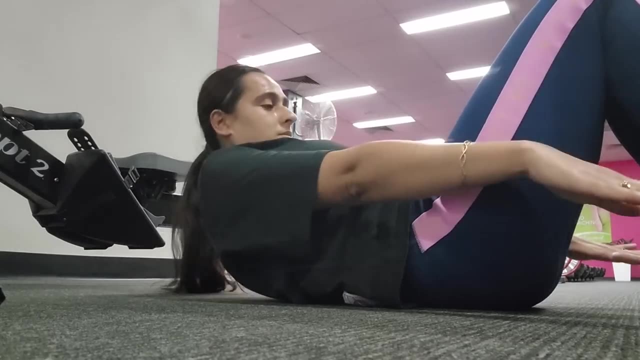 or simply assigning grocery tasks to my husband, and I took one responsibility off my plate, and this was a big one. It used to give me a lot of back pain as well, so now I'm more relaxed. as I know, my husband will take care of the groceries every week. 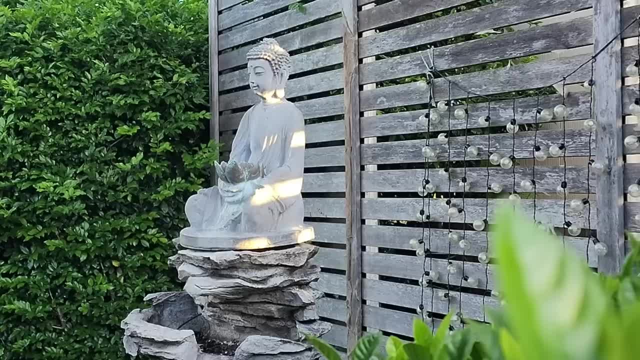 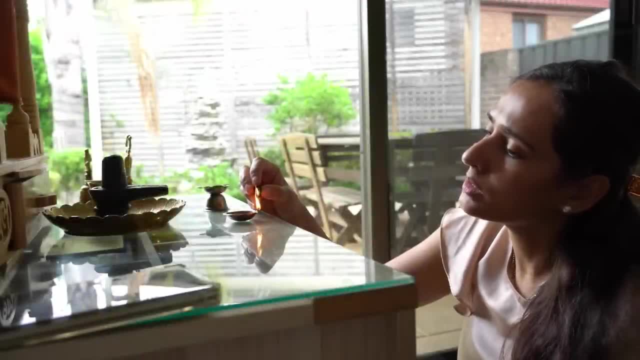 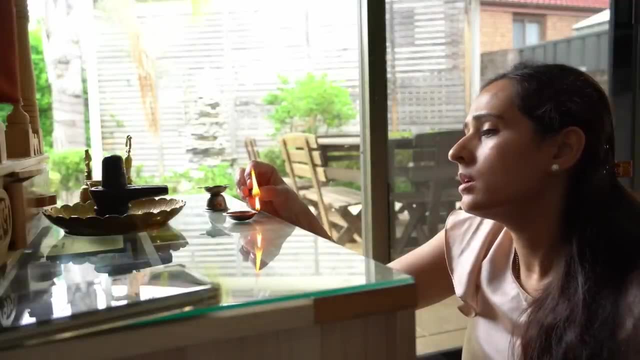 so I can spare more time towards my fitness or my another goals that I have set for myself. Third resolution is my spiritual health. well, sometimes some things happen in life that you get more attracted to spirituality. well, something similar happened with me as well, and one lesson that I learned that no one could help you in. 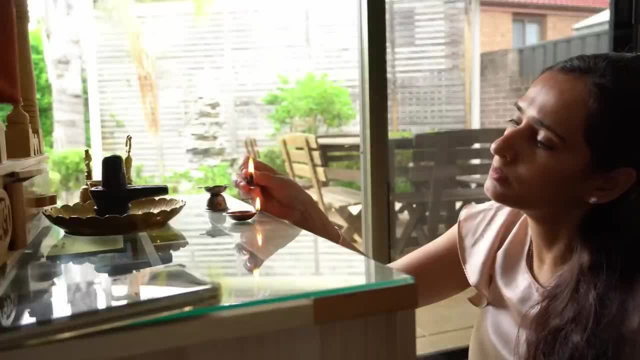 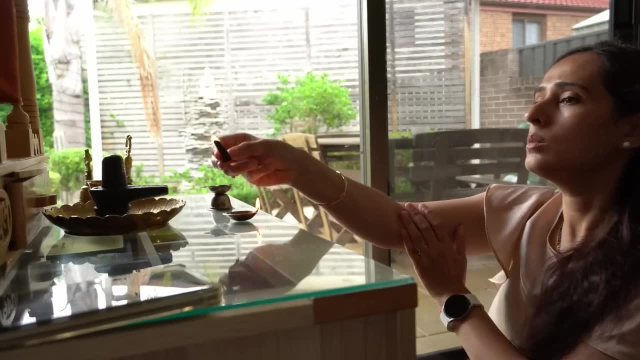 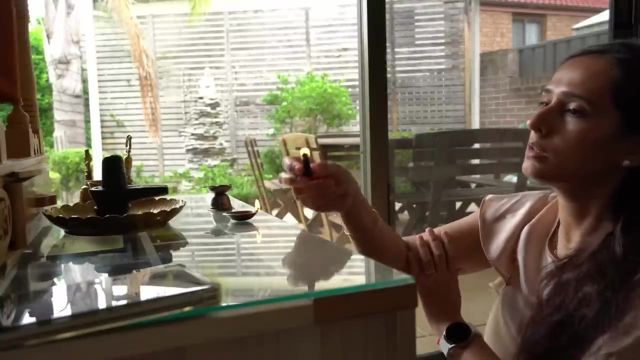 this life except God. He is the one who you should please, and not anyone else. Spirituality also gives you complete peace of mind, which you will not attain from anyone or anything external to you. Also, it makes you emotionally strong, and now you are not affected much with what people say or think about you. 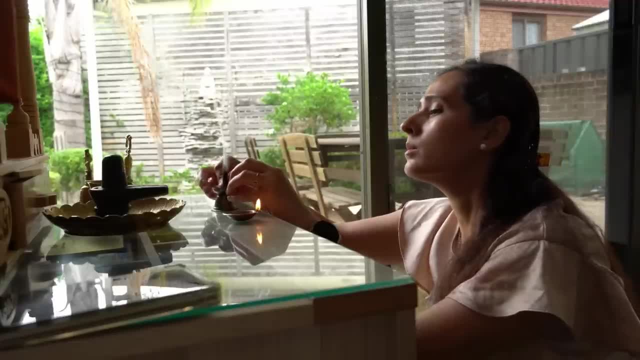 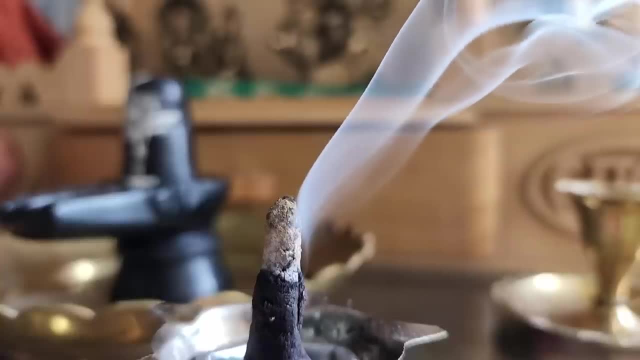 I have started doing Hanuman Chalisa every day, at least few times, and I am seeing amazing changes in my emotions. I am feeling much better and I am feeling much happier. There are few life lessons that I have learned over the years and I would like to share them with you. 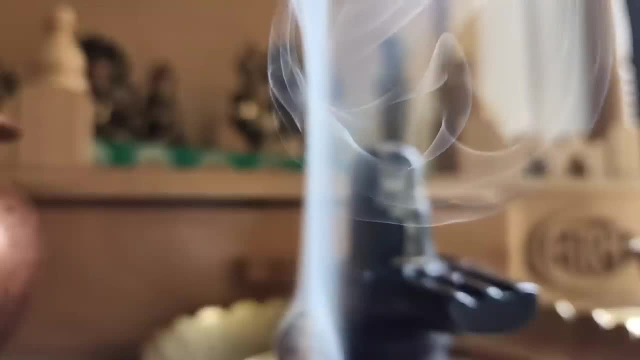 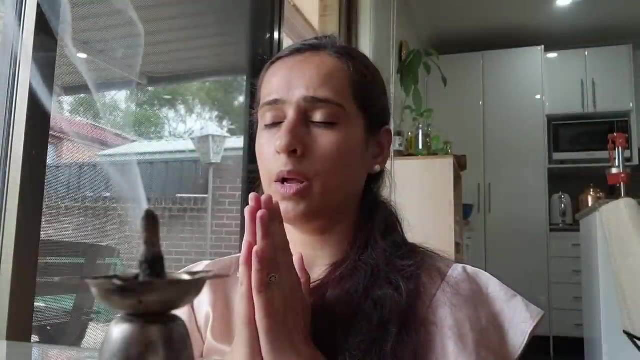 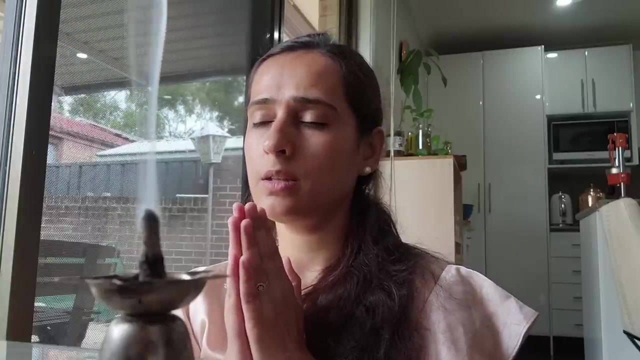 The first one being: do not hold grudges. It only ends up consuming you and not the other person. so let it go. It always reminds me of the frozen song: let it go, let it go, don't hold it back anymore, Anyways. the second one is: observe life. 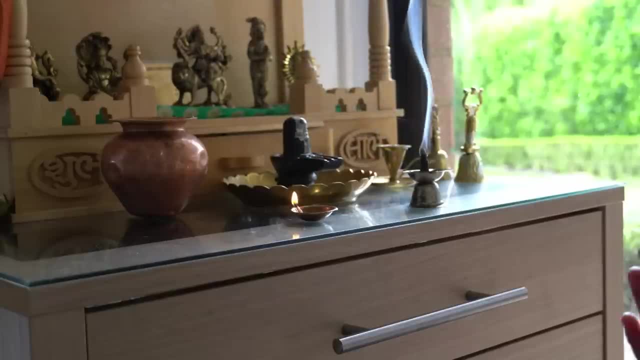 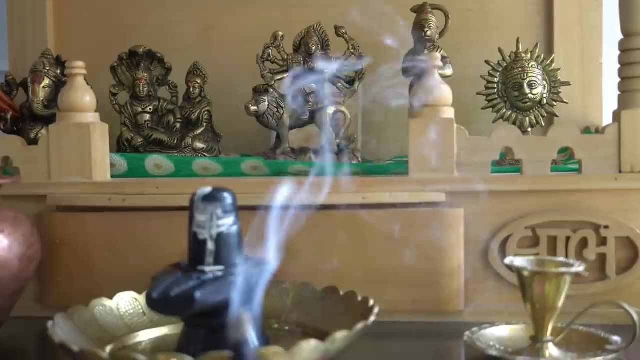 Do not absorb it, but observe it. Have healthy detachment, See everything be part of everything, but do not get consumed by it. The third one is meditation. Meditation cleanses your mind and gets rid of negative emotions, similar to how bathing cleans your skin and gets rid of bad odors. 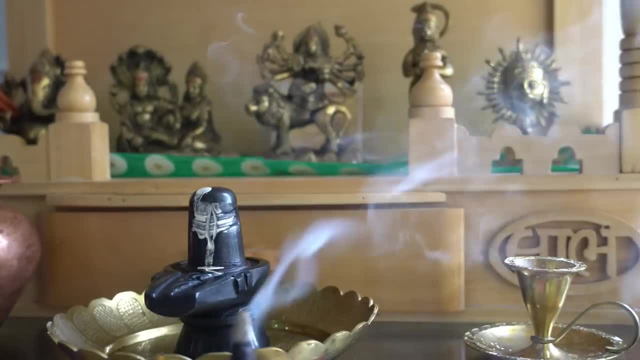 So, just like 5 minutes shower, do 5 minutes of meditation every day and you will have more control over your emotions. So, just like 5 minutes shower, do 5 minutes of meditation every day and you will have more control over your emotions. So, just like 5 minutes shower, do 5 minutes of meditation every day and you will have more control over your emotions. 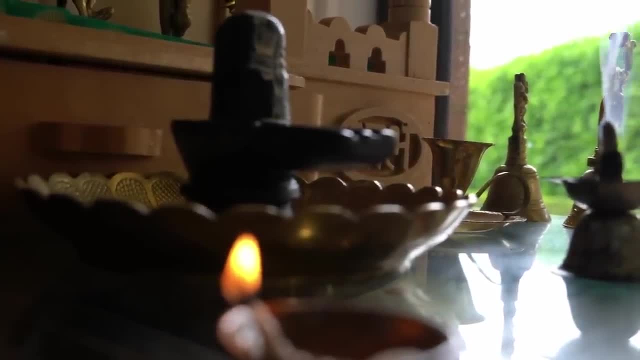 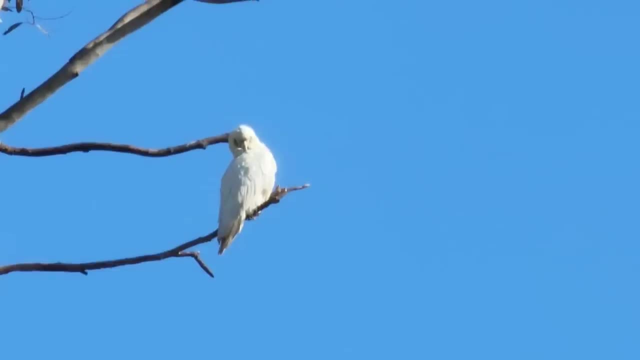 as you are clearing the bad energies, or the negative energies or emotions on daily basis, The last one being distancing yourself from people who do not value or respect you. It's actually a win, not your loss, So give these life lessons a thought. I'm sure there'll be many more life lessons that I'll be learning along my journey. 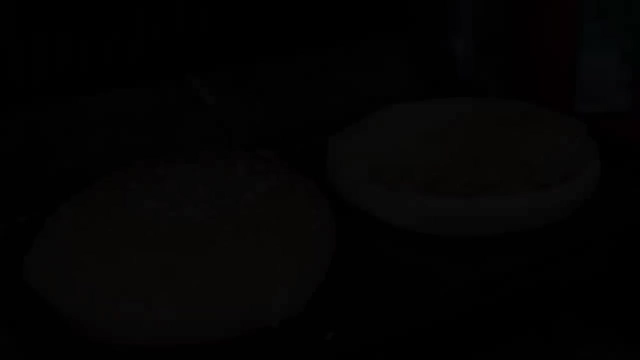 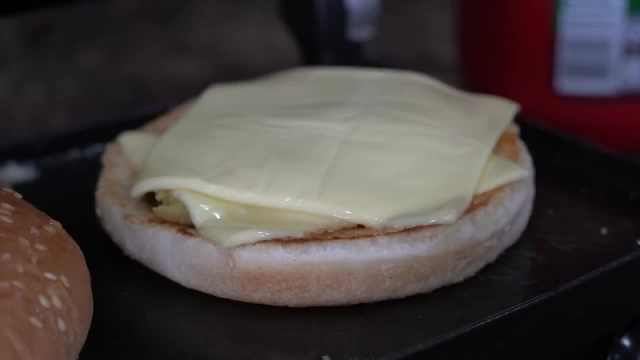 but these are few things that I always keep in my mind. These will only help you easier, But trust me, just like your husband, Your husband is like a golden lamb. He's just like a golden lamb to you. He will give back to you. 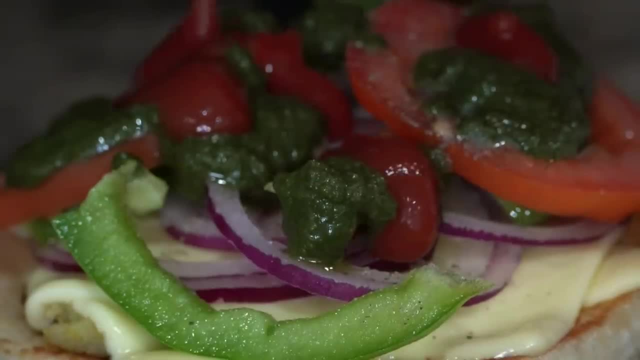 That's why your husband is the greatest burden to you. Yeah, he is. That's why your husband is the greatest burden to you. So you need to learn something new and you'll know what you've done well enough to be able to change. 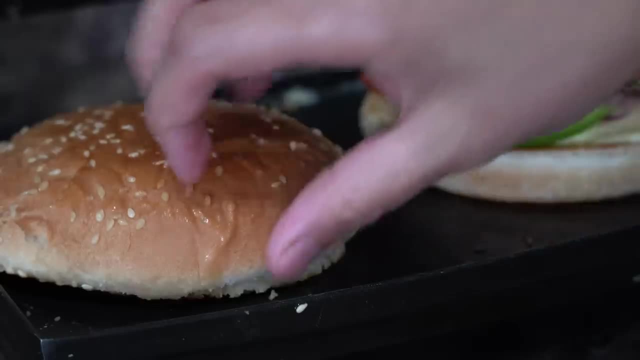 too. You didn't learn anything new in high school. Your job in high school is to be able to do something great at home. I know the pressure in your life is out of control. You know how you think your life is changing. You don't even have to teach yourself. 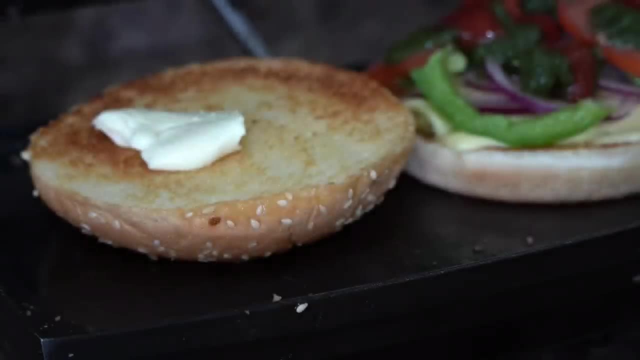 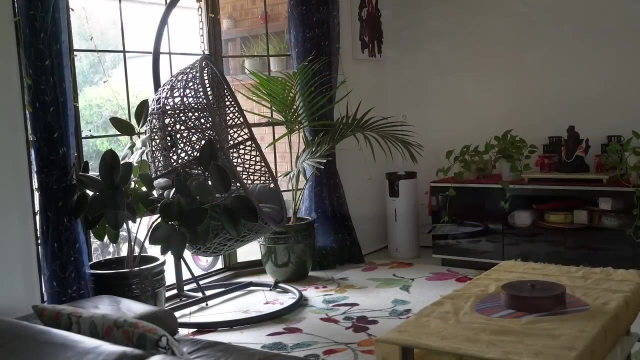 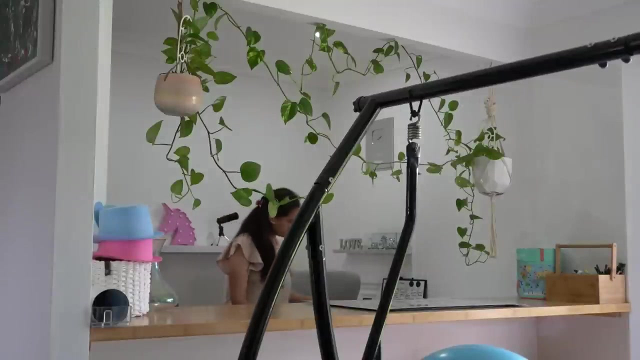 You just learn how to live your life, That's all. But the thing is, there's a lesson that you need to learn: to lead yourself. so last resolution is my financial well-being. as a girl, a woman, a mother, i can say that we. 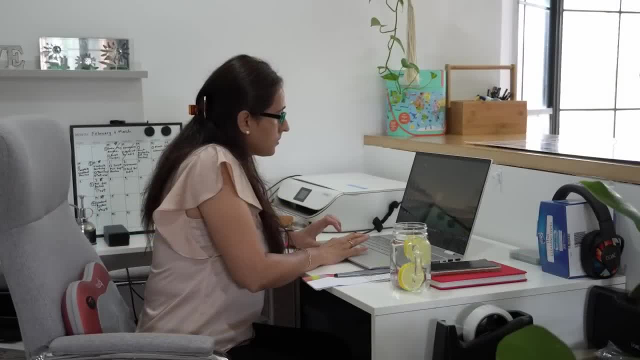 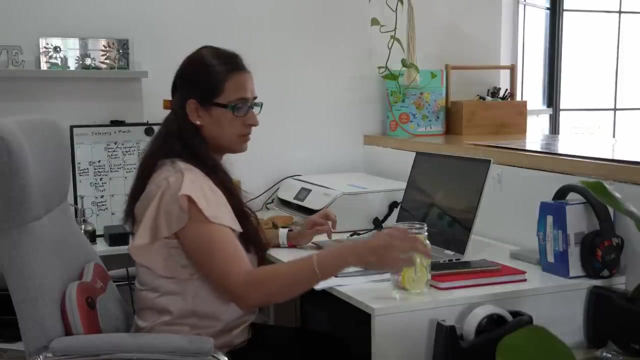 should be financially independent, as when you're in a bad situation in life, only your financial security will give you hope and strength. each girl should be financially independent, no matter you are a wife, a mom or a homemaker, as your financial independence is the only thing you. 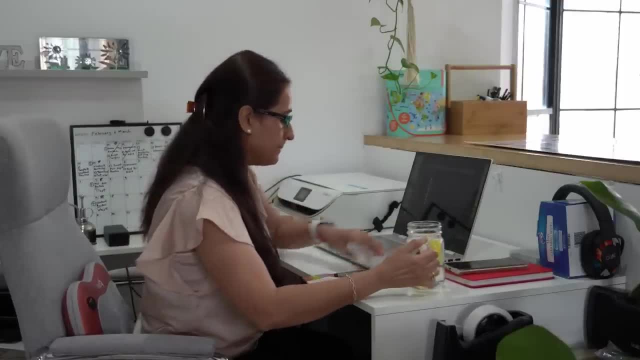 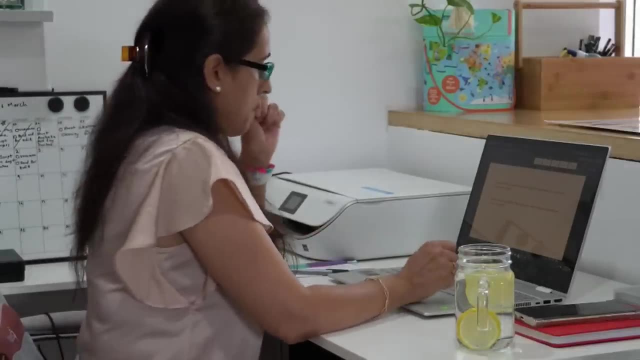 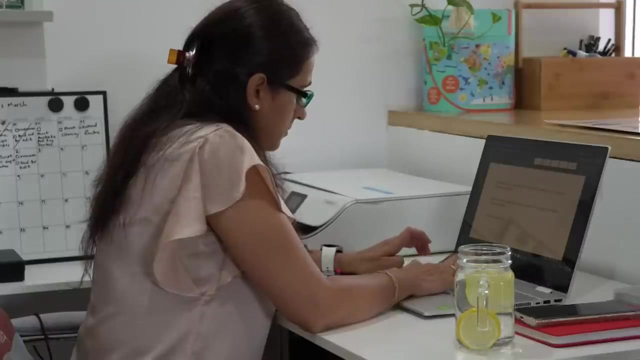 can fall back on. so i decided that, 2023 onwards, i want to make youtube a career, a priority, a source of income. i used to do youtube just out of interest, but now i want to take it more seriously and take it as a job, and my husband is in full support of this decision too. so now, after dropping 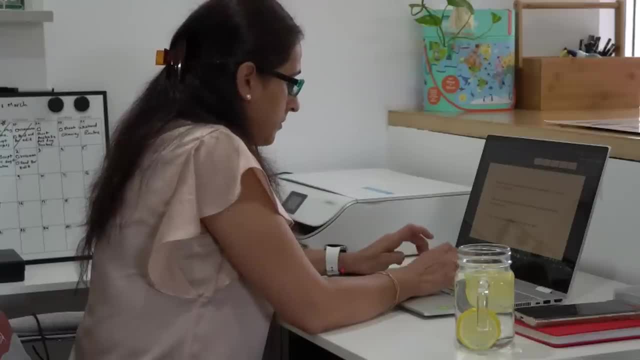 my kids. i go straight to the gym, as my physical and mental health is utmost important. i come back home, take shower and do my puja and hanuman chalisa, as my spiritual fitness is next important for me. then i will eat and sit in my office and work for two, three hours straight, till 2, 30 or 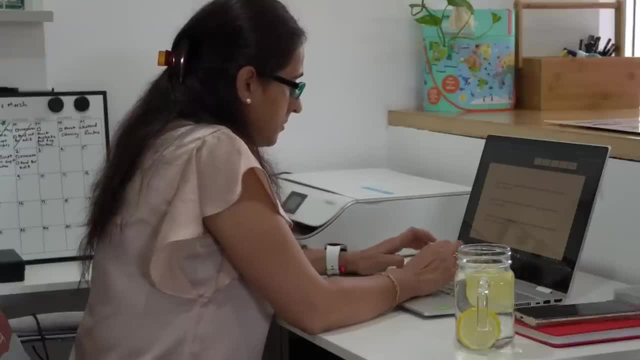 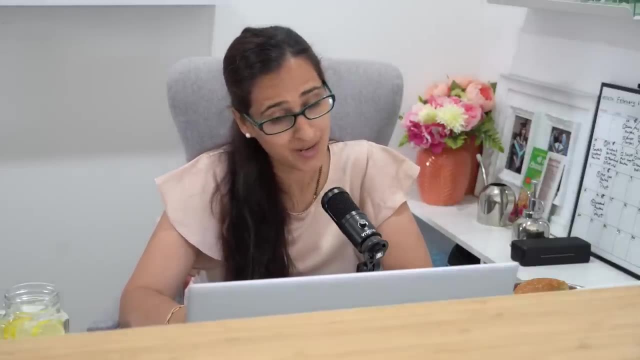 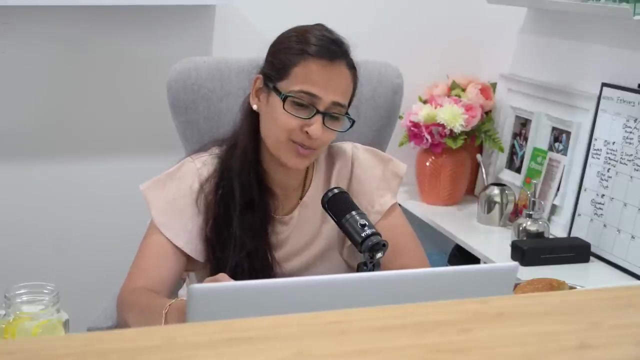 quarter to three before i go and pick my kids up. this is my part-time job, so when i am at work i think about pending chores, outstanding laundry. i do not take any calls, eat leftover food, do not worry about what to cook tonight or indulge into social media. my husband mentioned that. if you 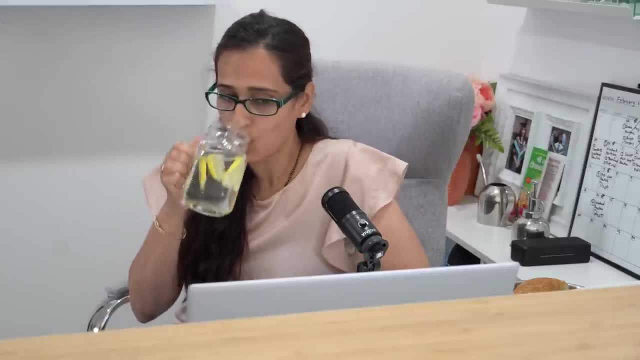 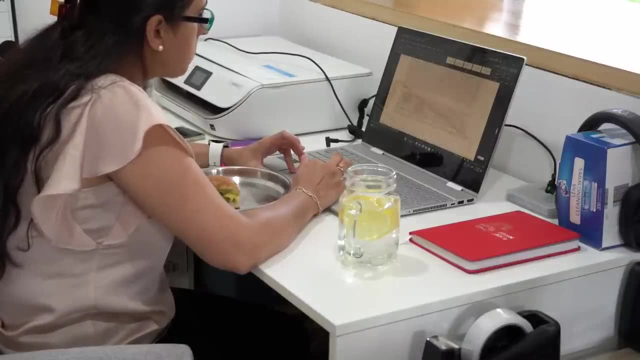 would be working at a firm or for some another person. would you actually drop kids and go straight to work, or rather come home to finish some chores? well, that thing stayed with me and that's what i follow. i forget about homemaking, about cooking, about what will be the menu. 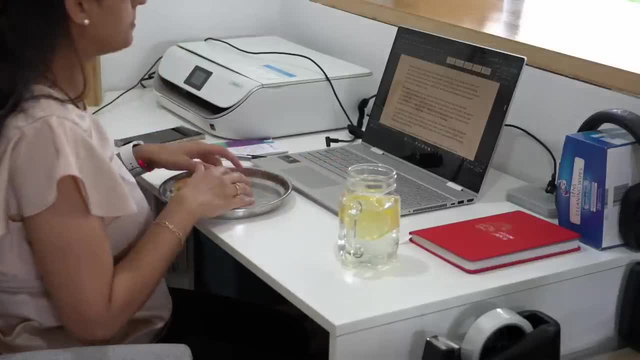 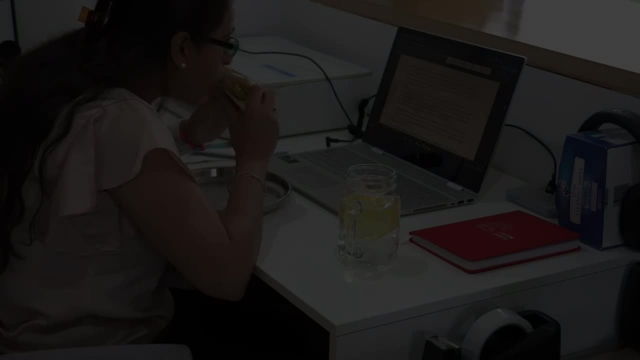 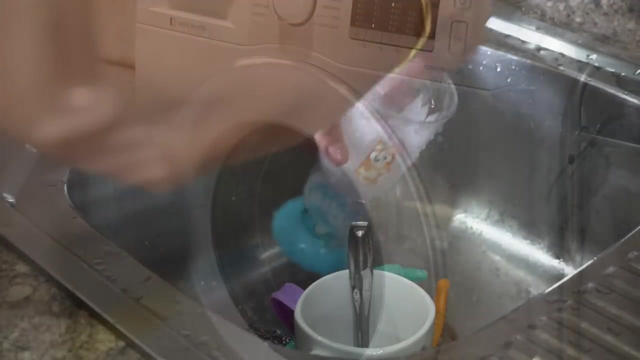 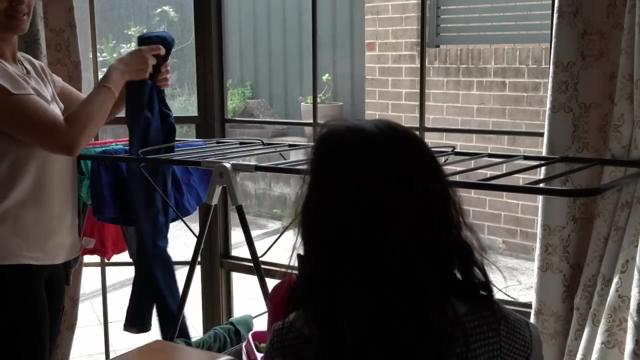 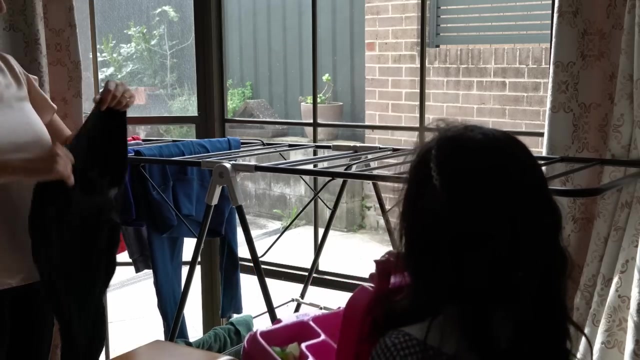 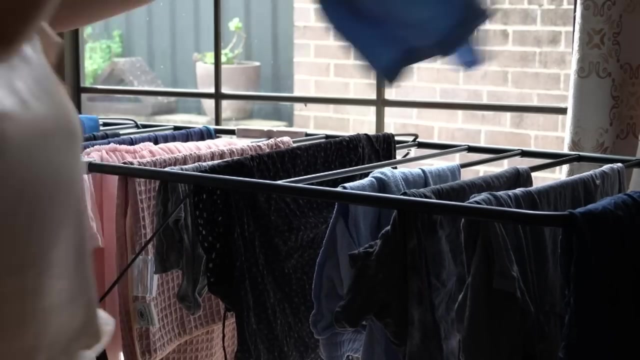 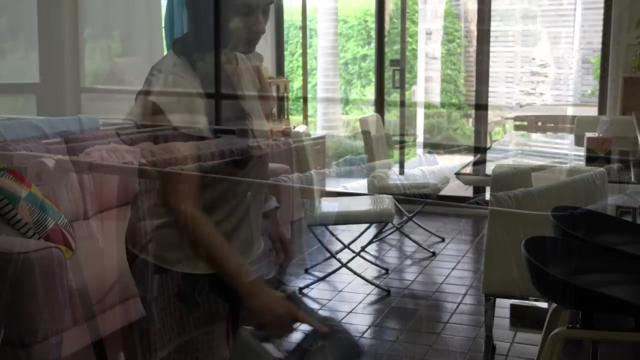 for tonight, etc. etc. and only focus on my job. and once the clock hits 2: 30, i get up, get ready, leave to pick my kids up from school. baby, acting like there's no tomorrow. acting like there's no tomorrow. acting like there's no tomorrow. 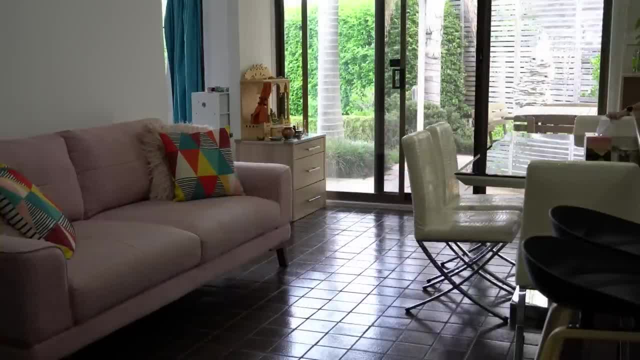 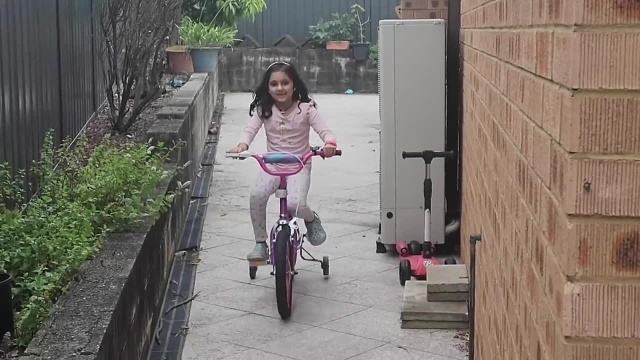 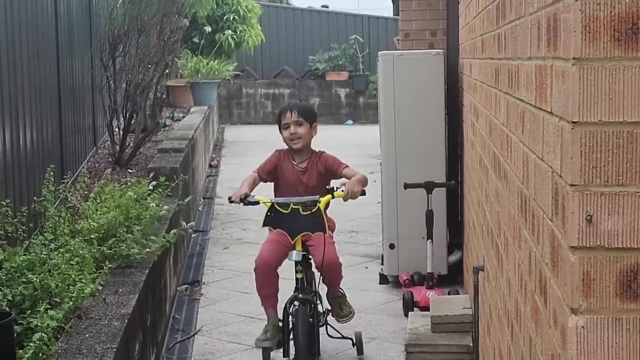 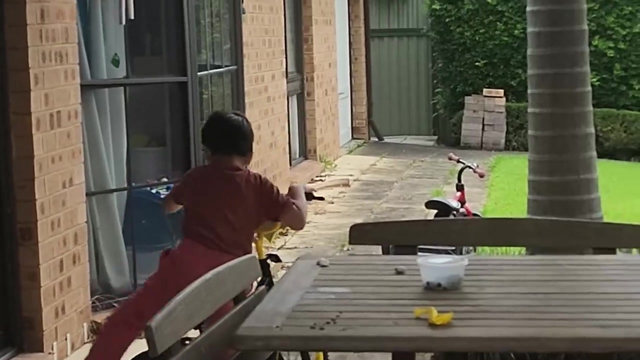 once kids are back home, i forget about my job and focus on my kids and home. so now i am not a working woman, but only a mom and a homemaker. i get kids started with the routine of showering or homework. they're free to play or ride their bicycle outside in fresh air, but not inside, as 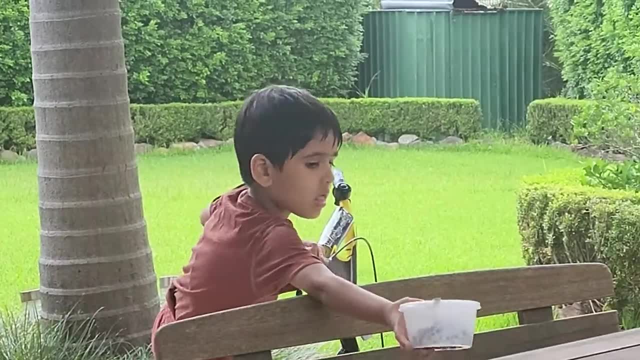 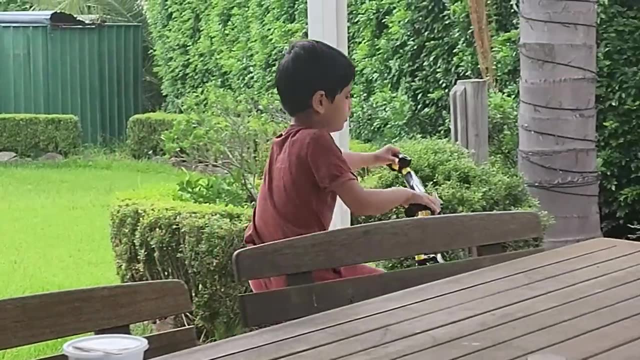 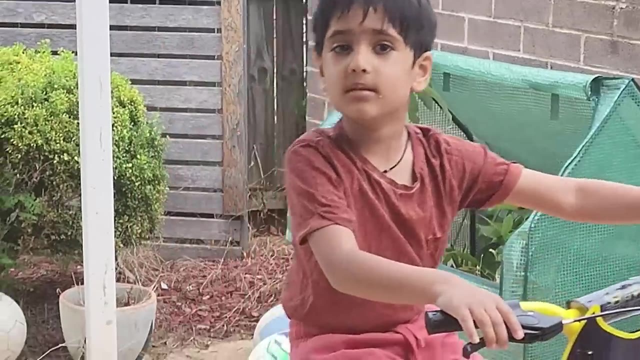 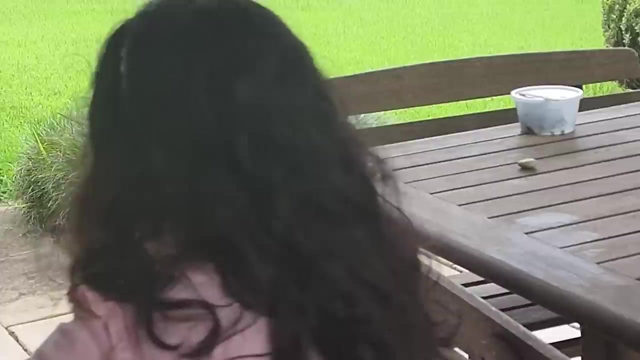 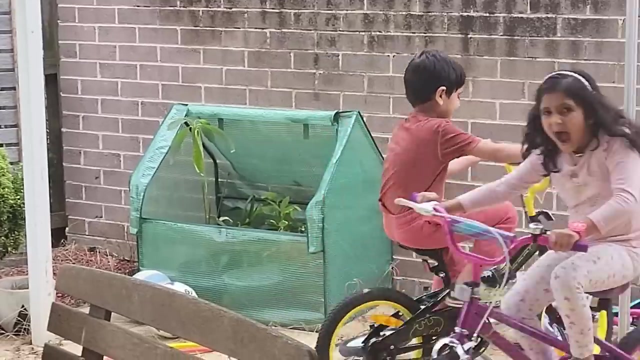 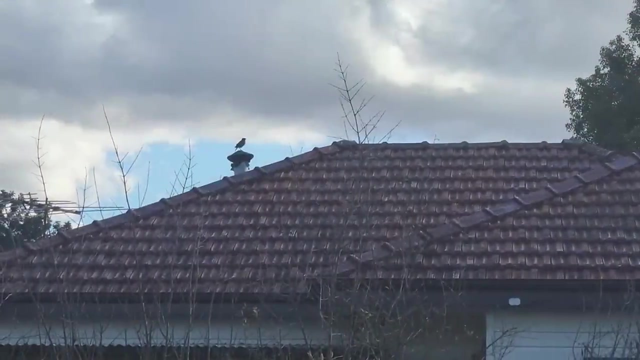 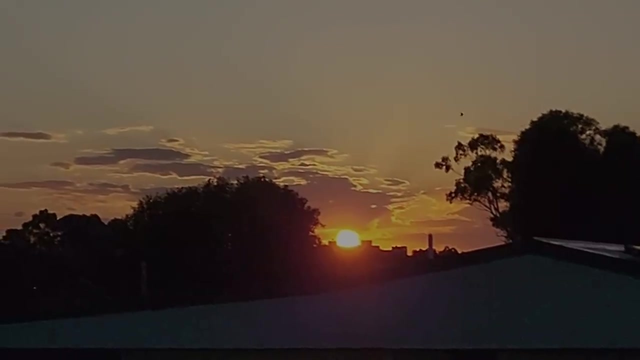 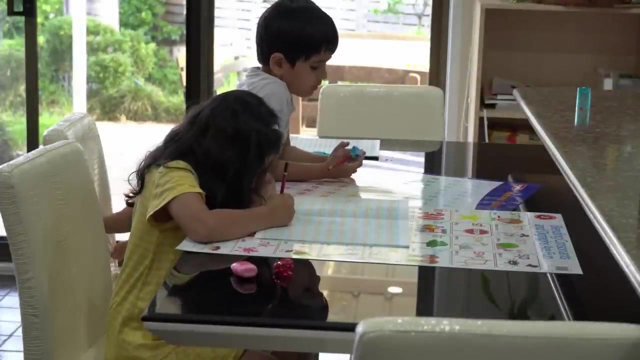 inside they only sit and do craft and make a mess. and also 60 minutes of physical activity a day is recommended for kids, so i encourage them to go out and play outside. once they are inside, i would sit and make them study for 30 minutes, as i want to get their 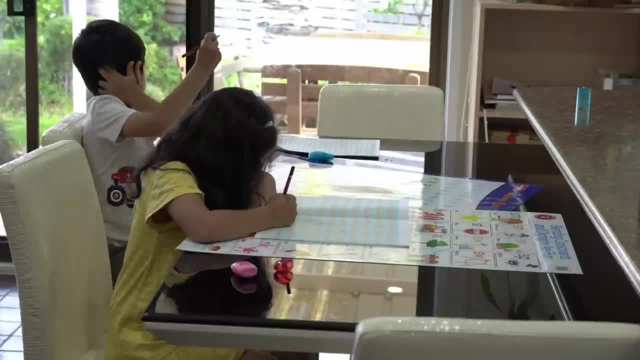 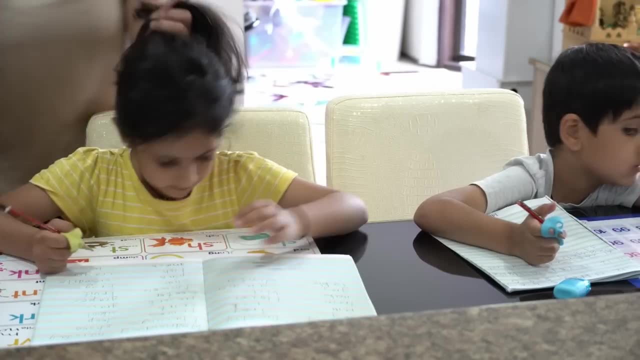 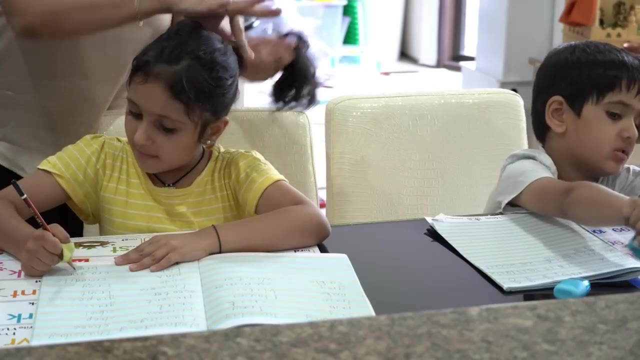 homework or home reading out of the way now itself. previously we used to sit and read at bedtime books and listen to music to learn about their family and friends. so now children are ready to go to school and take their shift and then on monday to thursday they sleep with their daddy. 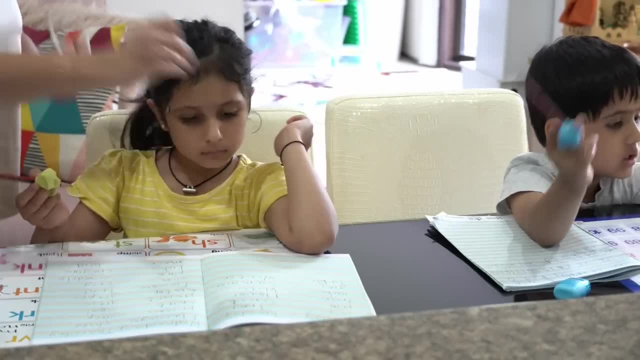 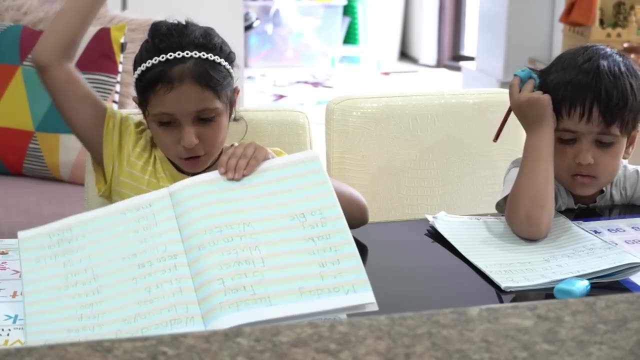 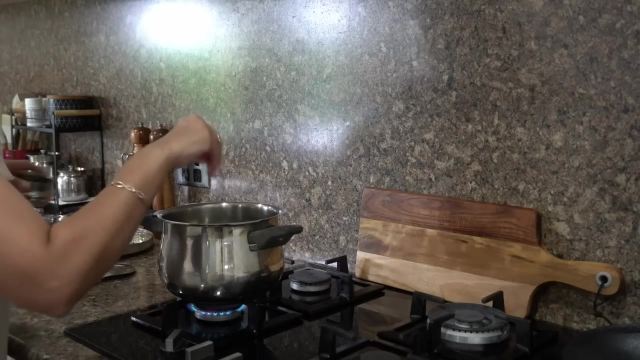 as i do my one hour of night shift after kids go to bed every night. i like to plan my next day, have it to do list ready so that i am up and running. this is quiet time, so i write down my thoughts, which eventually become part of my video like this one, and i share it with you all. 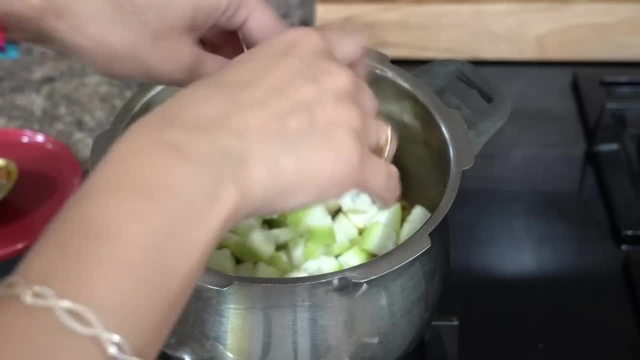 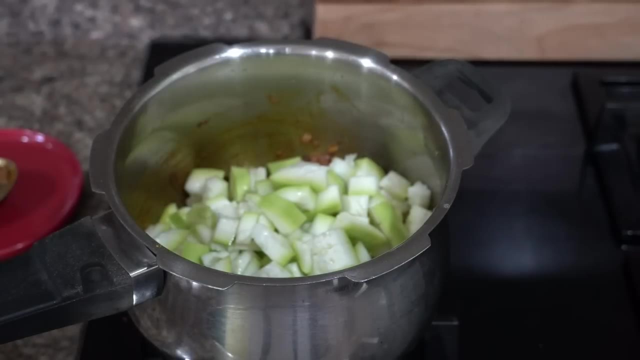 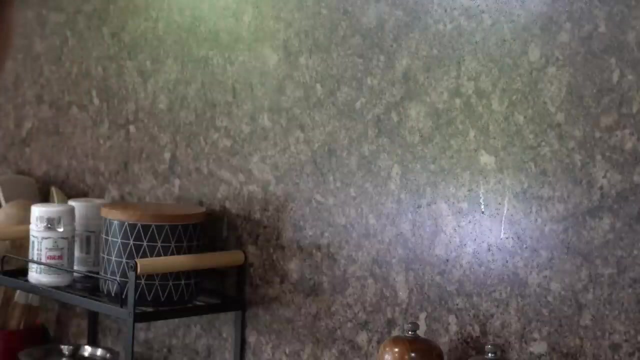 thing that only takes 30-40 minutes, as on weekdays, I do not want to spend a lot of time making special foods. Special foods and variety can wait for the weekend. Also, once dinner is done and dusted, I will clean up the kitchen plan on next day's meal. for dinner and kids lunch box I will 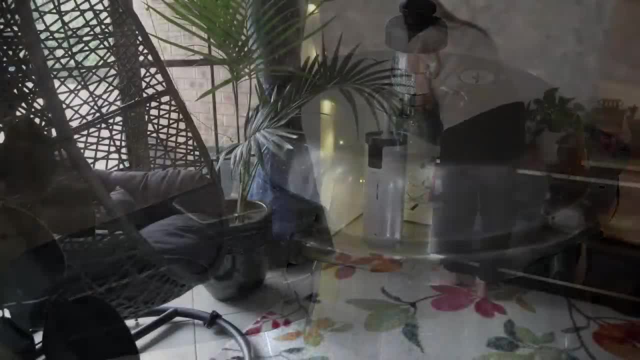 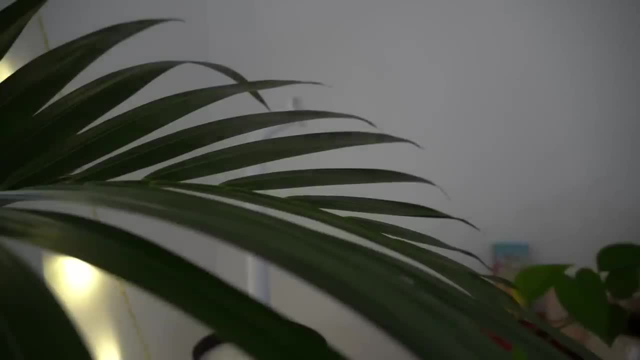 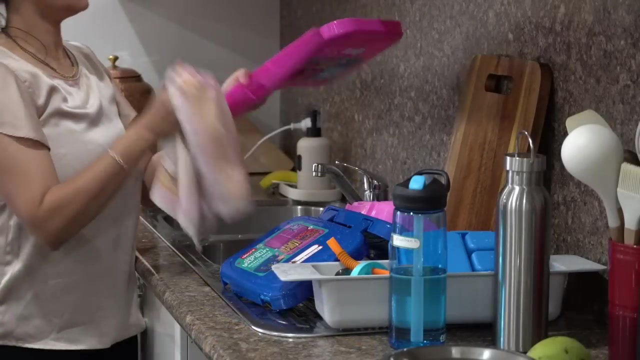 also rest for a little bit and do things that I love doing. Diffuser is one of them. I love to put essential oils in the diffuser and turn it on and just sit in between my plans, like you know, in my drawing room, and just relax. Once I'm done relaxing, I would go back to the kitchen and make sure my 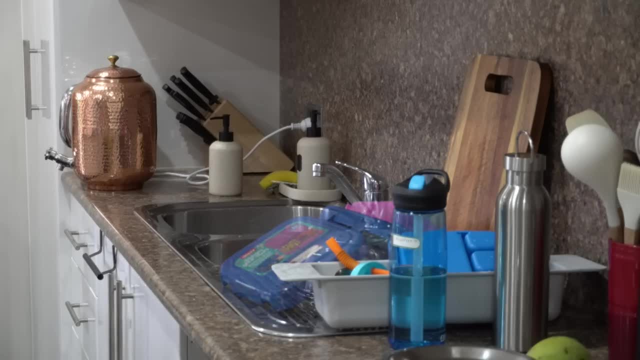 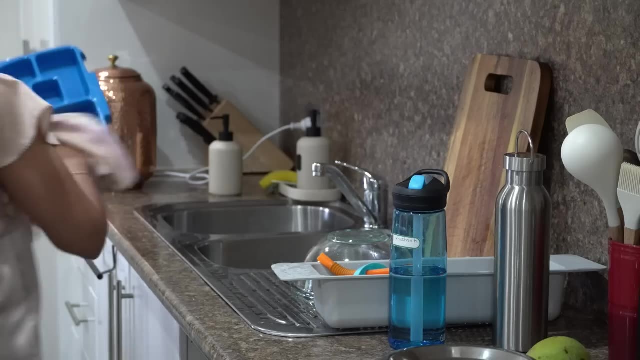 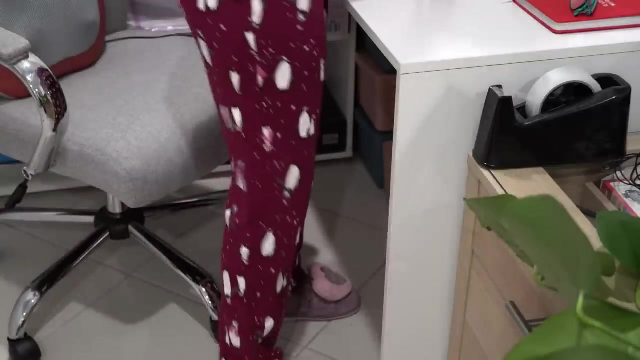 kitchen is pick a span at night, as otherwise dirty dishes will interrupt with my morning routine, next day and whole day. I will be lagging behind. So I reset my kitchen every night, so as I get a fresh kitchen each morning to work with. Now it's my night shift time. 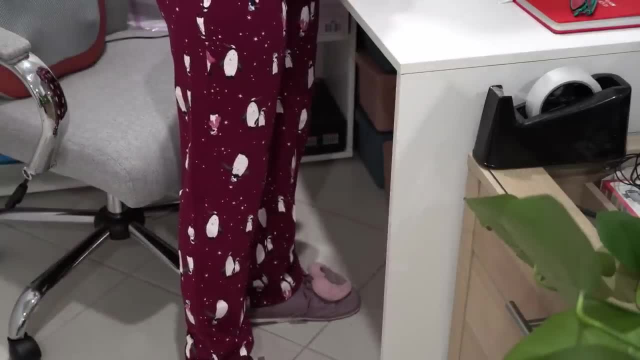 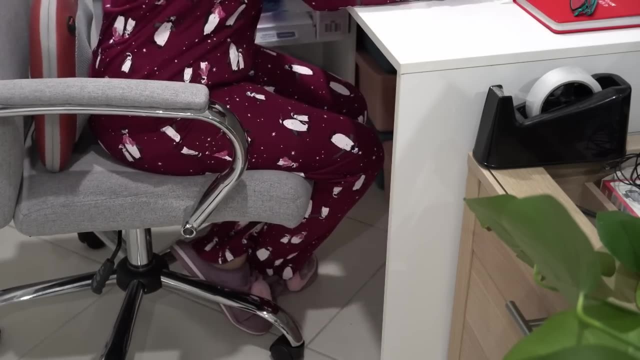 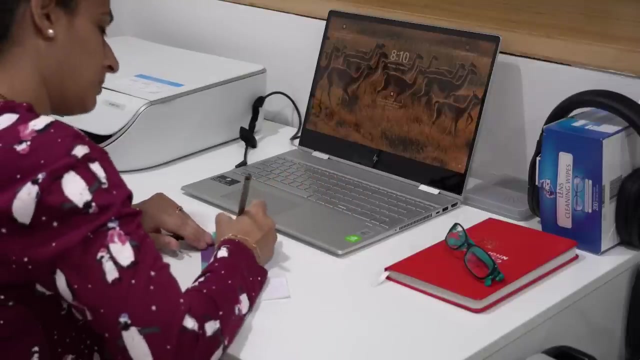 I am tired, but there is one important thing that I need to do, which is plan my next day. If I have a list of tasks on hand, then I have observed that my day is super productive and I can get tasks done at speed as well. So after kids go to bed, I sit again in the office and plan my work for the 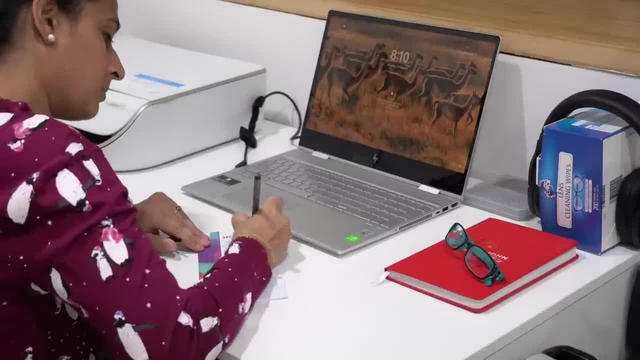 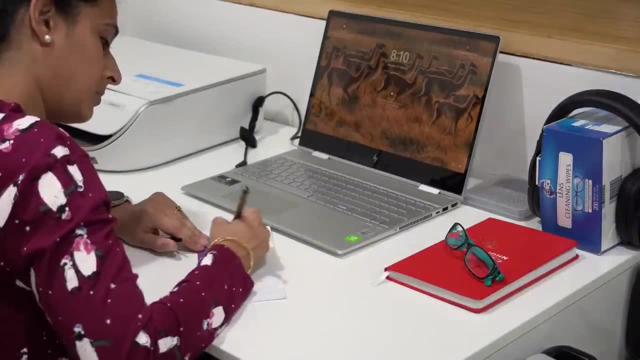 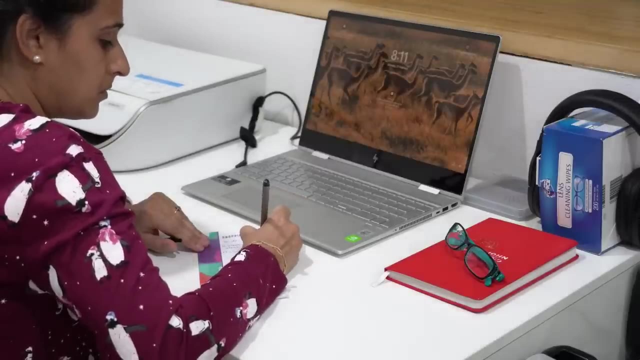 next day If I need to shoot, edit script, create thumbnail or description, or do I need to buy some supplies for the shoot, etc. etc. I write down everything. It helps me in two ways. One, it's off my head so I can sleep better and get a good quality of sleep. 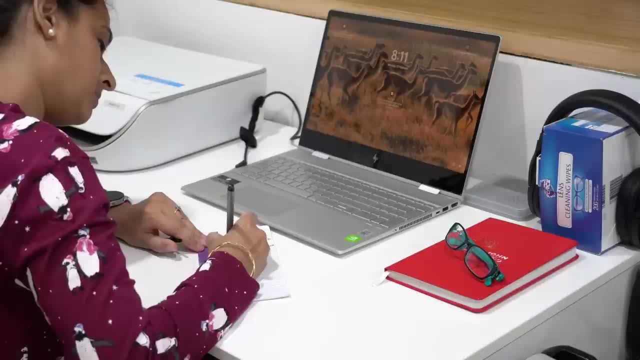 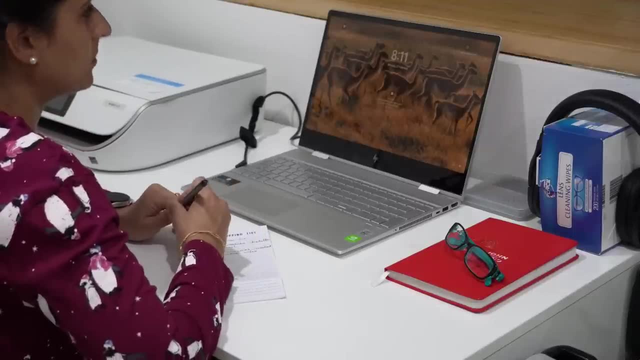 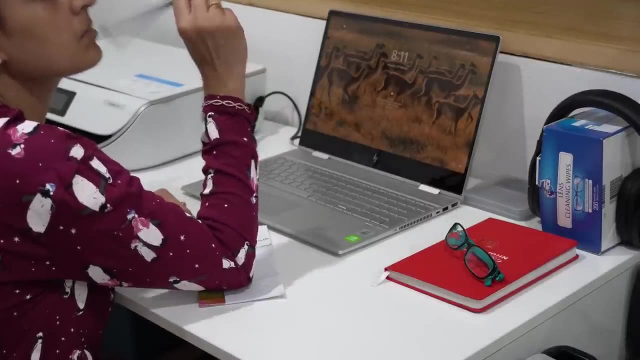 rather than just thinking about what needs to be done the next day, and have a light sleep or REM sleep. Second, having a to-do list makes my goals or the task concrete. I actually achieve them, as these are my action items for today and all I worry about is these items and not anything else, So I can focus. 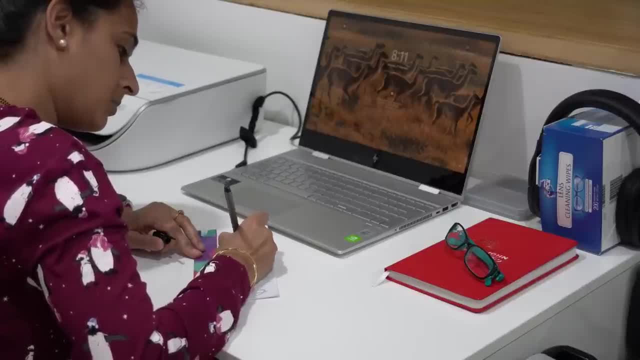 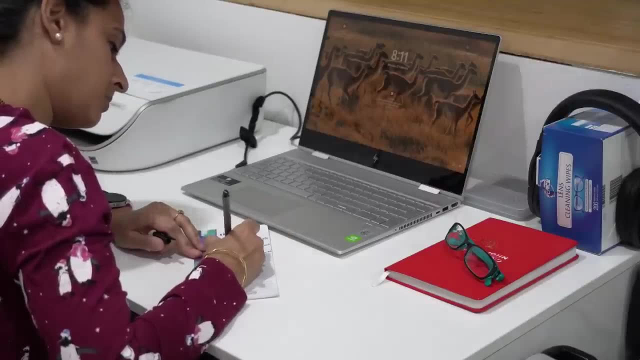 on them. By the time all these things happen, I am super duper tired. It's night time, It's around 9, 30 or 10 ish when I go to bed. but once I go to the bed I crash. I'm like I'm dead, not asleep, but another. 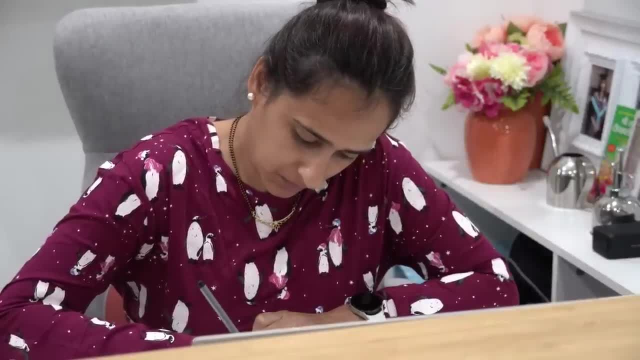 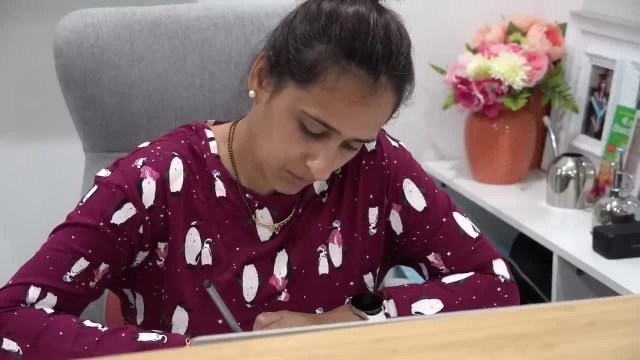 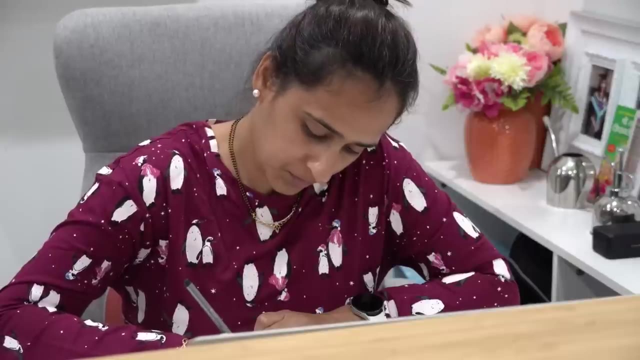 day comes, another start, another busy and productive day, and life goes on. So this way, I am working on my resolutions for 2023, step by step, day by day, and now, two months down the line, if I check my resolutions back, Yes, I'm working to achieve everything that I have put down on a pen and 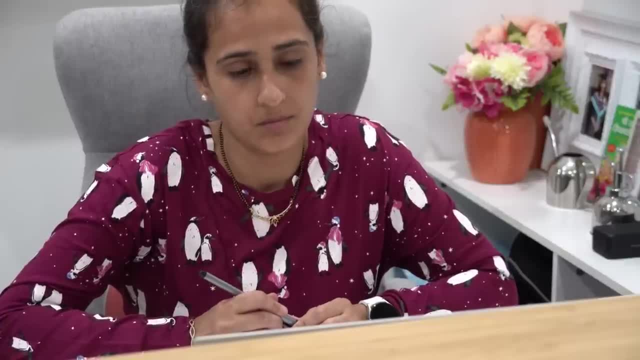 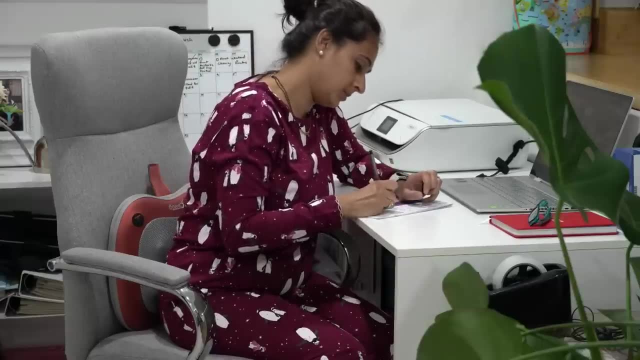 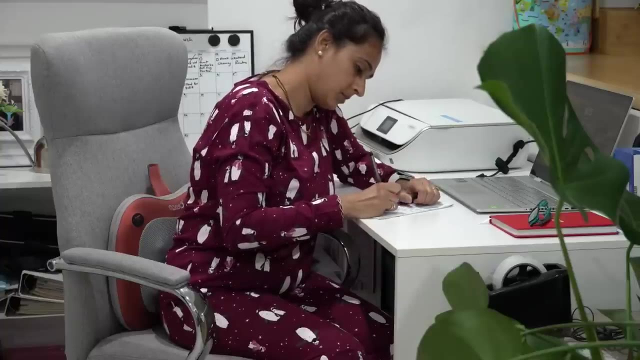 paper. I repeat, I am working towards achieving them and of course I have not achieved them yet. I want to go at a steady but consistent pace so that I can see results and not spend 30 hours in one week and not even spend like two hours the week after. Let's be tortoise and not a hare. 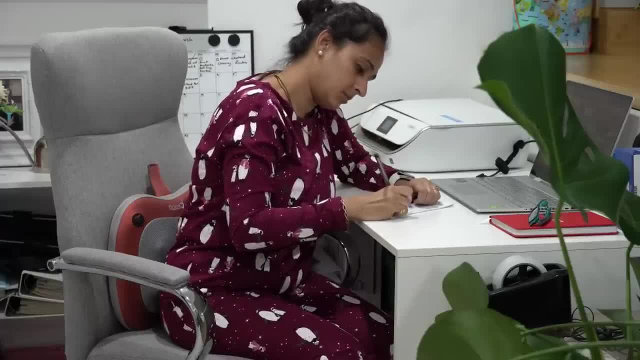 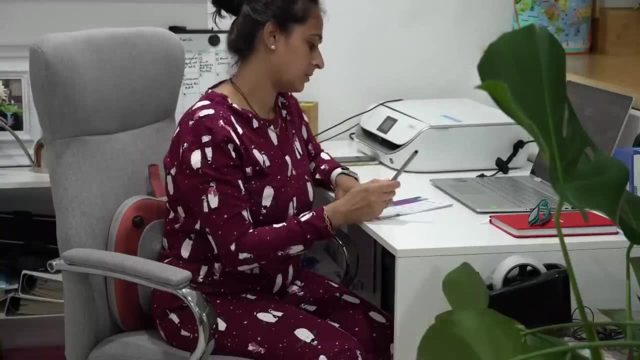 So, guys, my days are busy, tiring. Sometimes I do feel I have no energy, I do not want to carry on, but those days I take a break, I do nothing but sleep. Of course not sleep the entire day, but I take a good nap If I am tired. 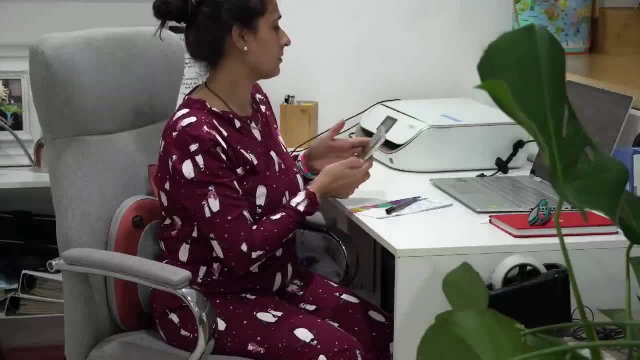 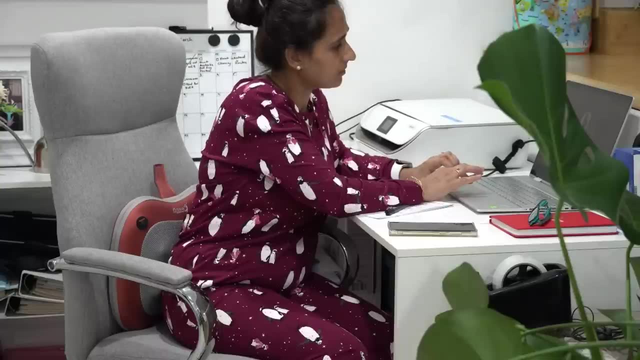 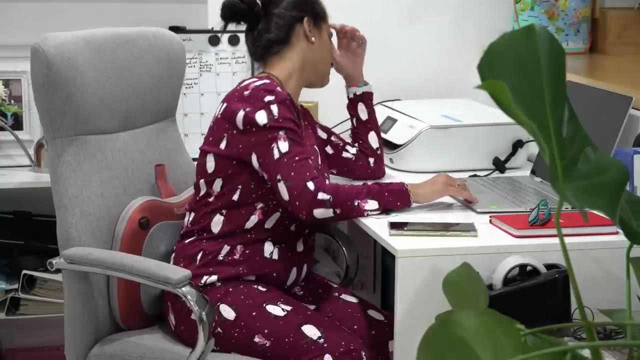 and stressed. I sleep that day, as sleep is the only thing that helps me reduce stress or recover from tiredness. I keep minimum contact with social media, as it only wastes time and gets you nowhere. Social media is not me time, but it's actually addictive and it kills time that otherwise would have been productive. 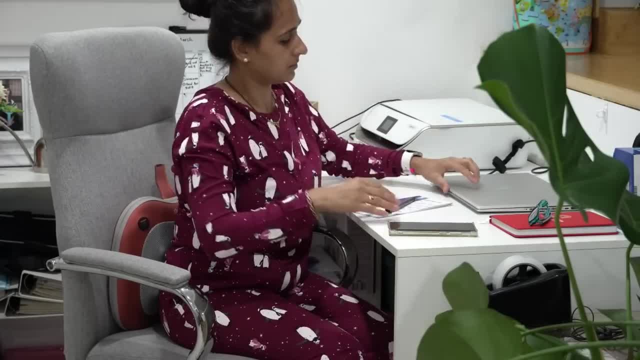 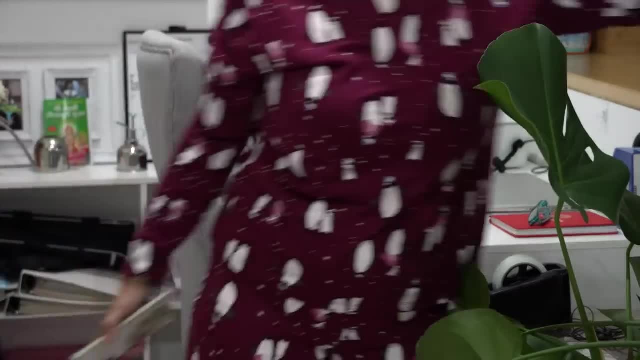 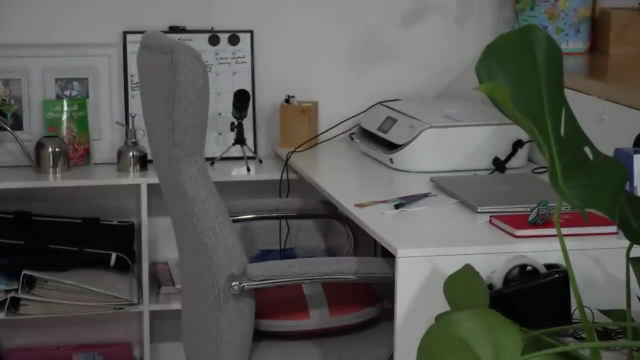 This routine has a balance of everything. I live as a working woman, I live as a mom and a homemaker and I love doing what I'm doing and would not like to change even a bit of my current routine for anything else. Routine makes you feel more organized and setting a consistent routine has 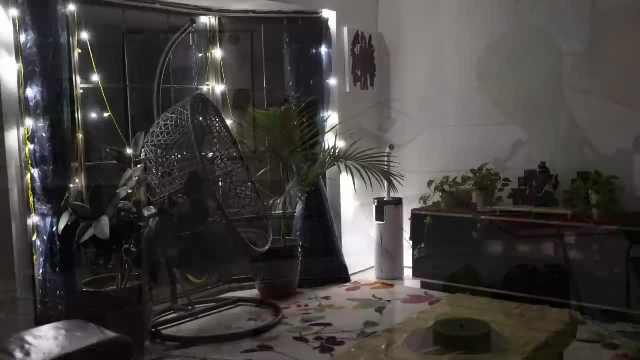 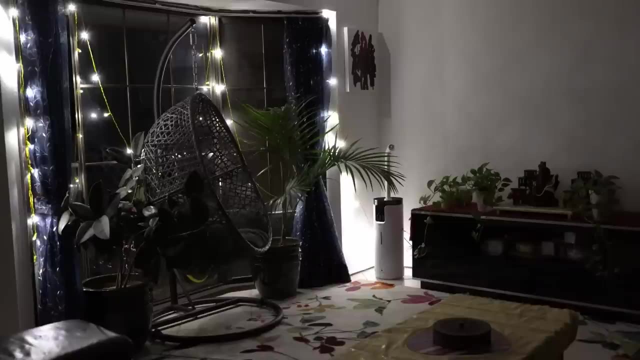 always been a struggle for me in the past. Now, so that I have this busy and productive daily routine, I wish fingers crossed that I stick to it for years to come and I finally see fruits of working towards my goal. So, guys, this is how my current routine looks like. but to achieve this kind of